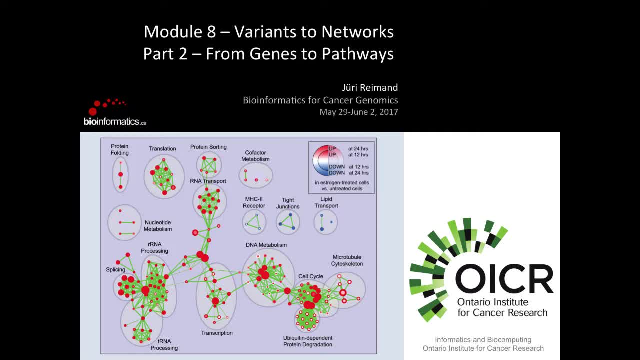 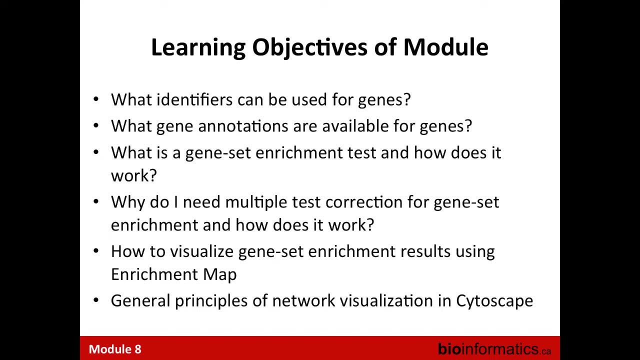 mutations tend to be sparse, and you can use the idea of pathways and networks to group together meaningful variants into biological themes. Alright, some of the learning objectives of the modules. Genes have many names and it can be a complex maze to navigate, so we need to understand how to use identifiers for genes. 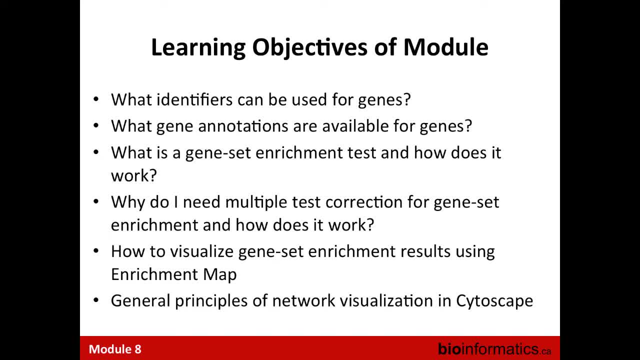 and how to convert those identifiers. Also, genes have been studied. They have been studied to a greater or lesser extent over the years and therefore they have many annotations. from these studies We have ideas of what genes may be doing and in which cell or compartment they may be acting. 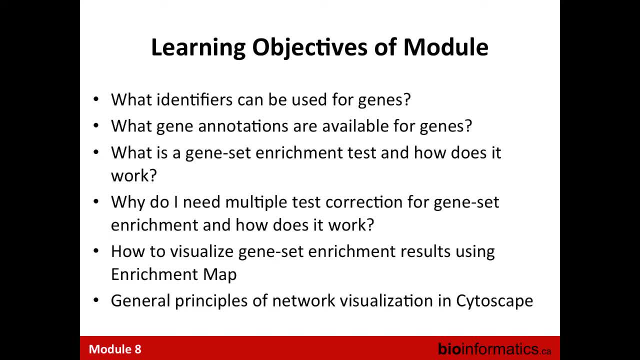 Then we will learn about the gene set enrichment test and how we would use it for our purpose of interpreting genomic data. Then we will learn about multiple testing corrections- and why would one use a multiple testing correction? And then, finally, we will learn about gene set visualization. 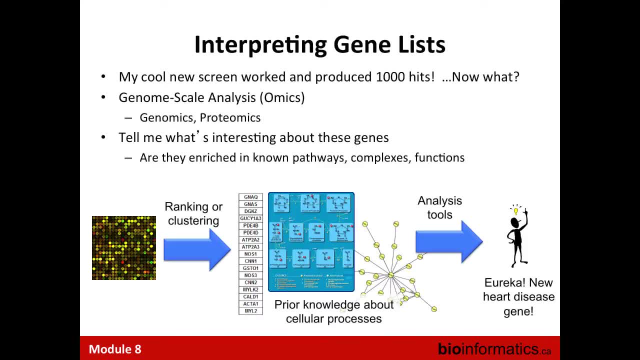 And finally, we will learn a little bit about enrichment math. Okay, so this is a very classical scenario in the era of high throughput biology. You do a cool experiment, or maybe a sequencing assay, and you come out with a thousand hits. Now what? 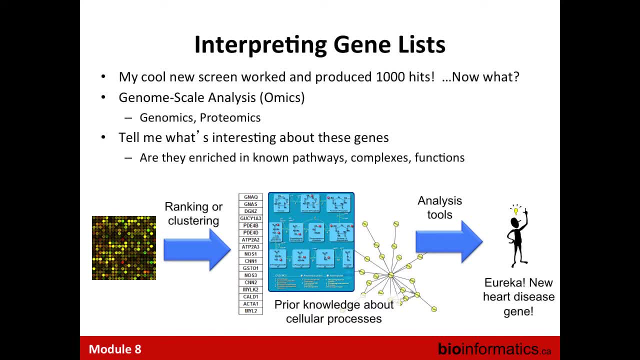 You don't really want to analyze these hundreds or thousands of hits one by one, And what you usually do is you perform some sort of statistical or mathematical analysis. You come out with a thousand hits, You do a ranking or clustering of genes and end up with these long lists of genes. 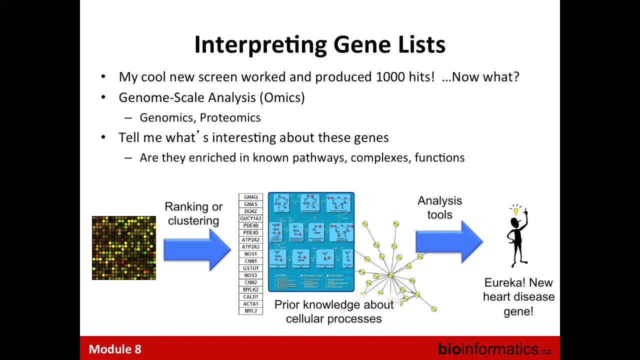 And to further, better interpret your long list of genes from your experiment, you need to use prior knowledge. So genomic databases, pathways, networks, literature, and you better use this with different analytical tools because otherwise it's a hassle and in the end you will maybe find: 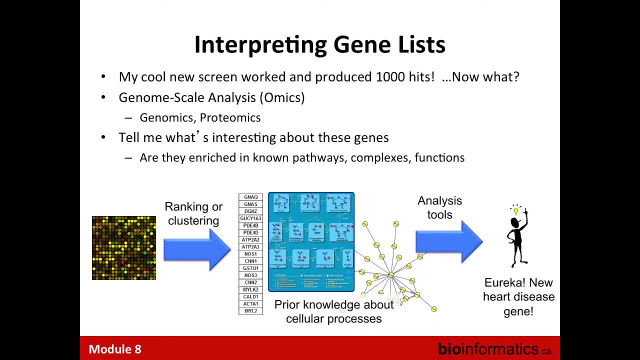 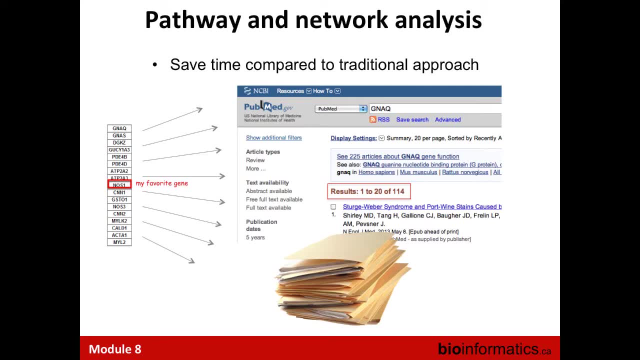 something new about your favorite molecular mechanism or gene and you publish a good paper. One way of doing this is using The PubMed database. so you have a hundred genes of interest. Each one of them will have maybe ten associated papers. Some genes are famous, like p53 will have a hundred thousand papers. 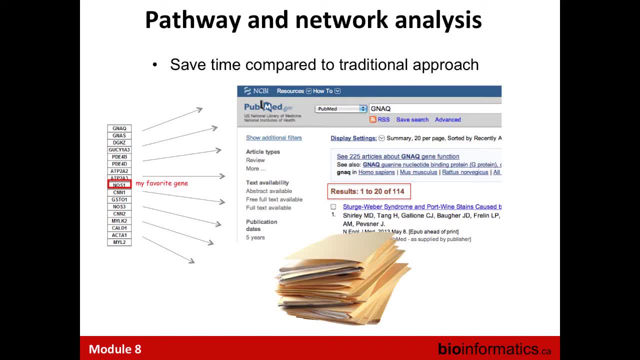 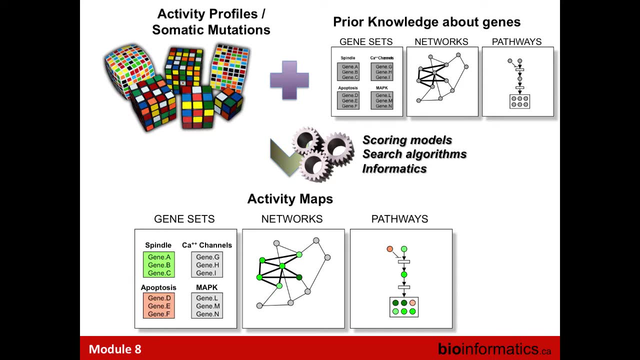 And then you just do a little bit of reading one by one and you'll eventually end up in the same spot. but maybe you don't have all the time in the world to do that, So this is why you want to use pathway and network analysis tools to do this in a slightly 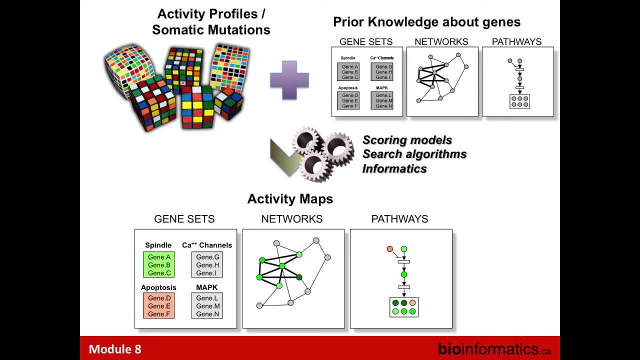 more systematic way, in a statistically sound way, and come up with a Faster solution. So pathway enrichment analysis in the way we describe comprises two major components. On the one hand you have genomic activity profiles, which is a very broad way of saying anything that you can measure in a high throughput experiment. 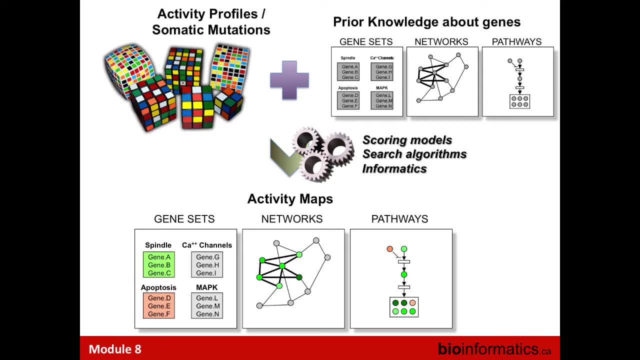 For example, you could measure all the somatic mutations in a set of tumor samples, or you could measure the gene expression, the profiles of all the genes in the cell. So you'll get maybe a list of genes or maybe a ranked list of genes. 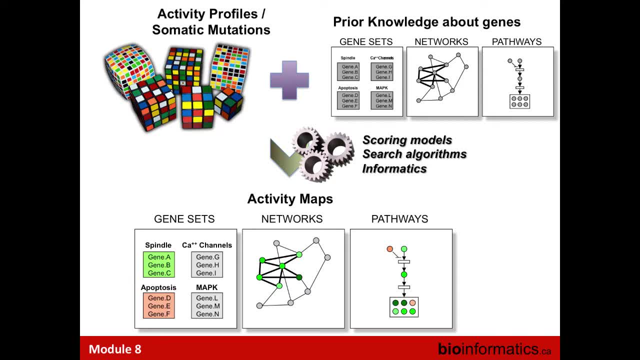 Or perhaps genes with scores, And on the other hand, we have abundant knowledge about what genes have been doing or have been observed to be doing in various experiments that have been accumulated over years and years of research in various pathways, pathway databases and network databases, and genomic 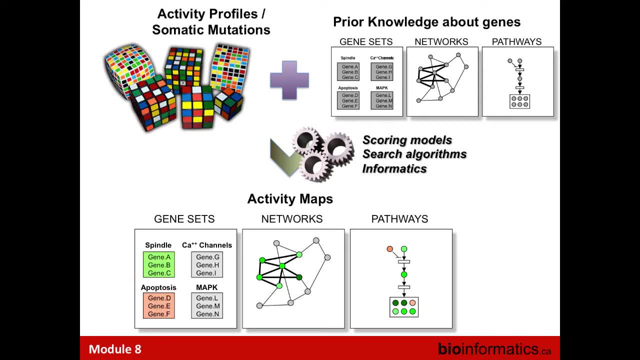 databases. Using these two sets of information, so gene annotations and the gene themselves, you can use various tools that statistically integrate gene information annotations and then you come up with, say, pathways or networks that are enriched in your genes of interest, or maybe some structural relationships or gene regulatory networks, and so on and so forth. 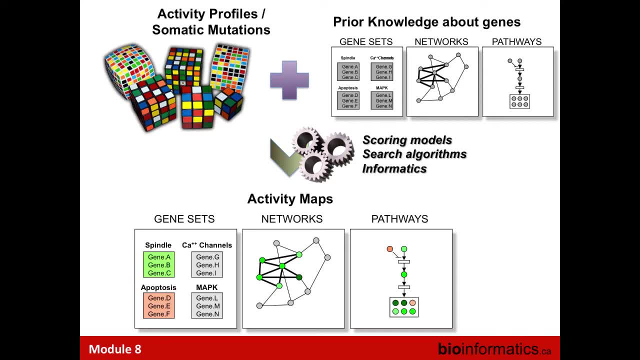 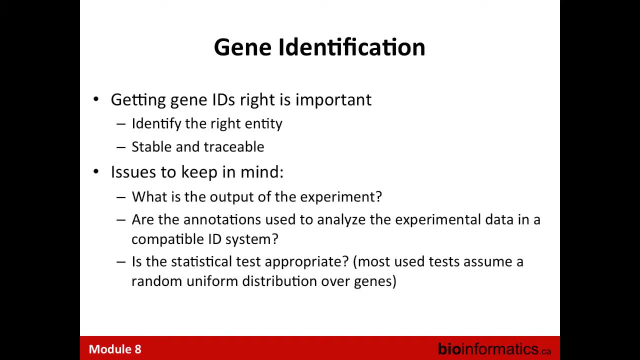 So this is a very general description of a family of methods that can be applied. But before you go into that analysis, you want to call genes with the right names. This is really important because there are increasing, you know- even meta studies showing how. 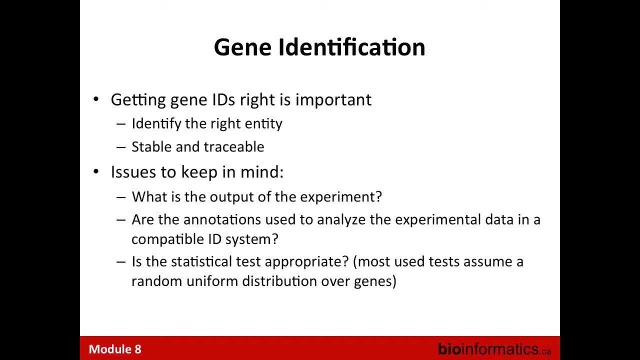 one's favorite tool, the Excel spreadsheet, tends to generate the wrong names just by opening up text files, which apparently affects up to 20% of scientific literature in high impact journals, which is? It's scary, right. And besides these very obvious things such as Oct 4 being converted to October the 4th, 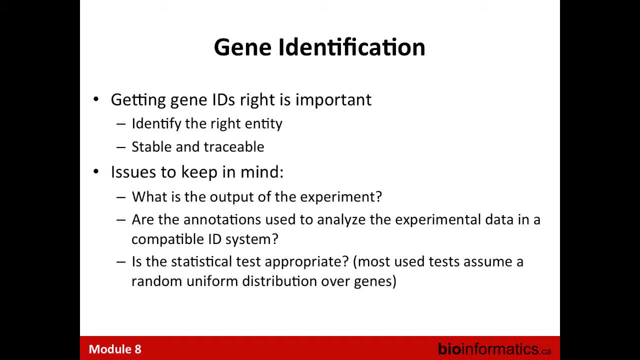 there are other, more subtle things. because people have studied genes over time, They have tended to call them different names, and these different aliases and names still float around, And this is very, very common in the genetic community, And so there are many conditions that can cause confusion in your bioinformatics pipelines. 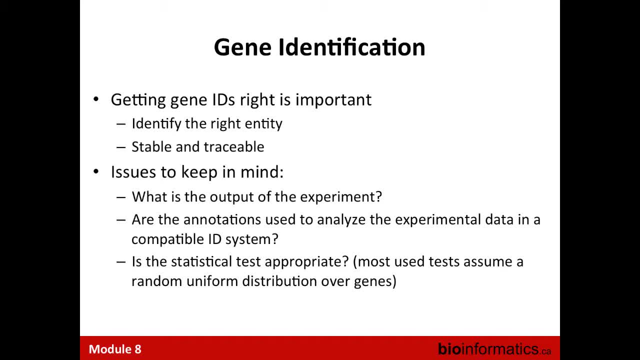 Also, different genomic databases call genes according to their own identifiers And often there is no clear one-to-one mapping between them And these issues. that you want to keep in mind is also that your genomic experiment handles some sort of IDs. Perhaps you did a microarray experiment? 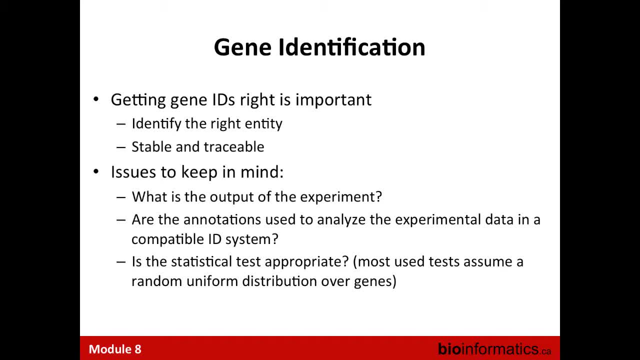 Microarray probe sets come with their IDs. When you map these probe set IDs through the genes, there is no one specific gene that's going to identify them- one-to-one mapping in many cases- and you want to use automated tools to do that. 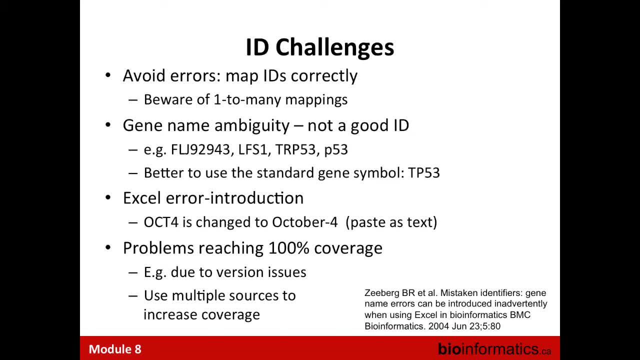 And then, moving on to some of those IT challenges, one of them is one-to-many mappings, particular identifiers corresponding to multiple genes, the identifiers that have been assigned over time. People who speak about genes sometimes don't talk to people who talk about proteins, so 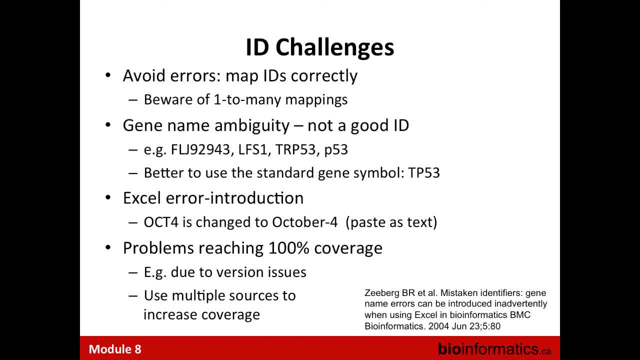 gene identifiers and protein identifiers are not overlapping. and then there are these major efforts to bring everything together. For example, the gene symbols are supposed to be a standardized set of genes that are unique. However, even the gene symbols from the Human Genome Nomenclature Committee, they change. 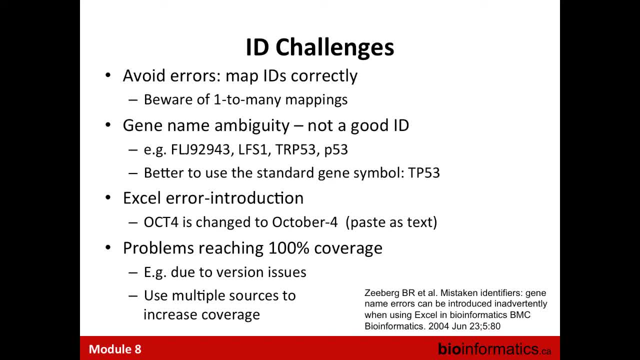 about 10 percent over a few years, as we just found out. Error introduction: I just mentioned October 4, the stem cell regulator is a very important example of this, but there are other examples except two, And there will always be problems of reaching 100 percent coverage of all the genes in the 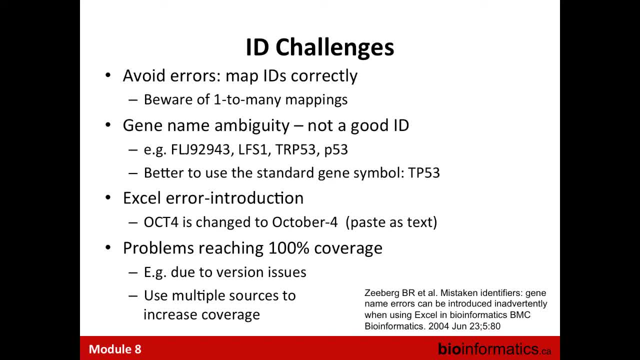 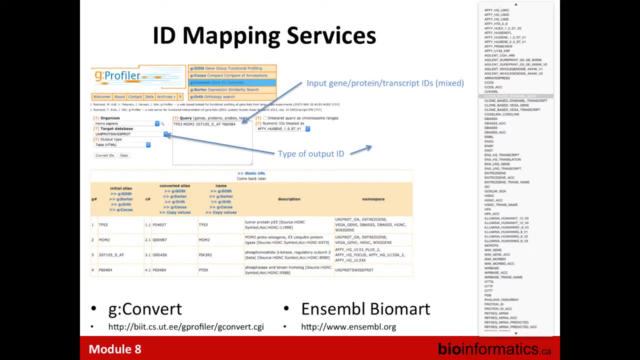 genome. so if you really want to achieve that, you should go through these examples one by one and perhaps try different resources- gene cards, ensemble, UCSC- to make sure that the gene that you are talking about maps to that and identifies multiple sources. 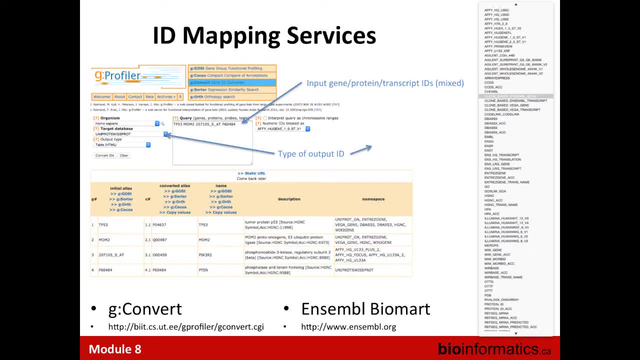 There are automated tools that do ID identifier mapping for you. The first thing we are going to do is set up a specific mapping for a gene. This is a well-known example, but there are others that accept it too. This is part of Gprofiler. that's part of my PhD back in the days. 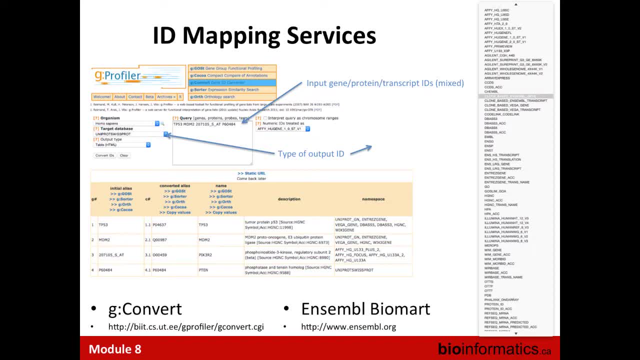 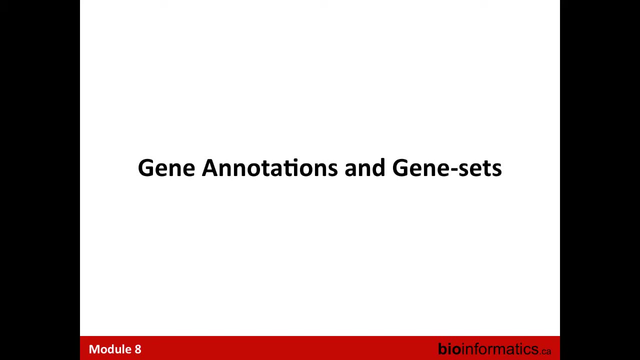 It's called GeneConvert and it allows you to convert a set of gene identifiers to various different sources, And there's probably a few dozen different types of identifiers that are supported for each species. For humans, it's more than a hundred. Now let's imagine that you mapped all your gene identifiers and you're happy with the gene set. 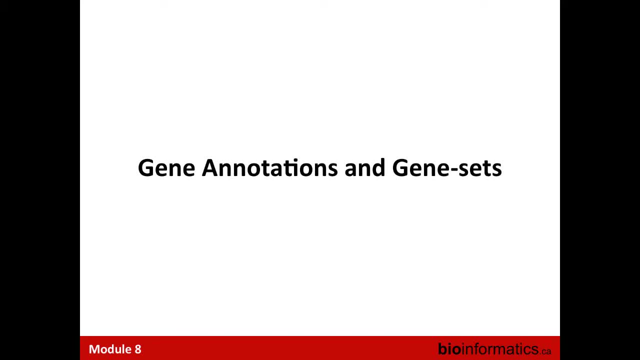 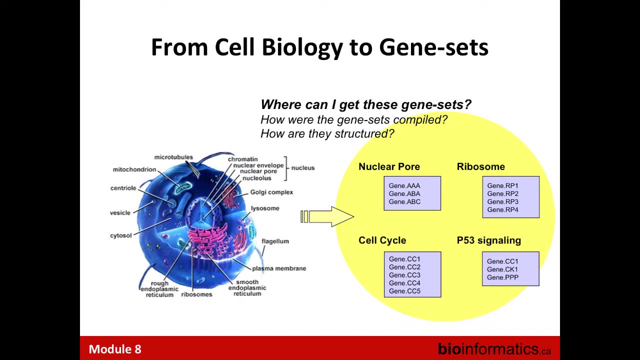 You need to start interpreting them in the context of pathways and networks, And pathways and networks are really abstractions of cellular systems and biology. So here on this slide, on the one hand you'll see like a pretty three-dimensional picture of the cell. 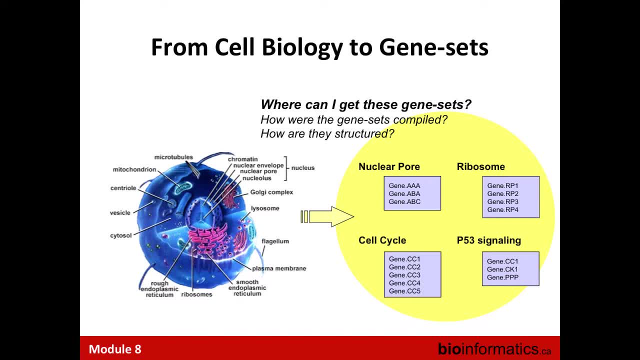 And on the right-hand side of the slide you'll see the database description of that cell. as far as we know, using our current knowledge, So various components of the cell, various processes of the cell and molecular functions ultimately boil down to this. 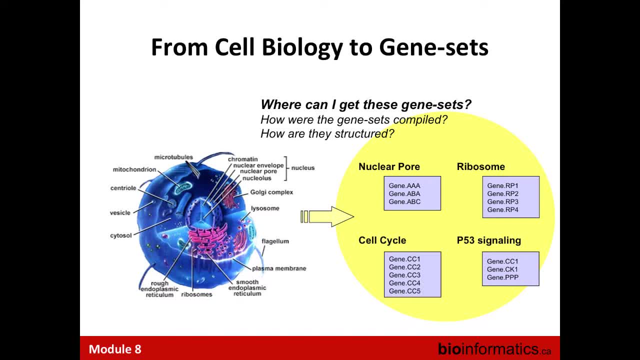 This is the simplest type of a pathway or a functional characterization of biology, Just lists of genes associated to some sort of function, tagged with a particular term or a description or a sentence. Obviously, this is much more complicated because genes interact with one another. 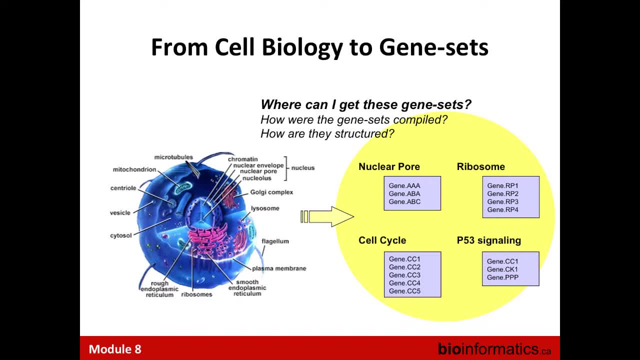 They activate or inhibit one another or make physical complexes. But in the most simplest form, when we talk about functional anatomy, we just talk about gene sets and gene lists. Are different genes in different lists, Like is one gene going to be in different lists? 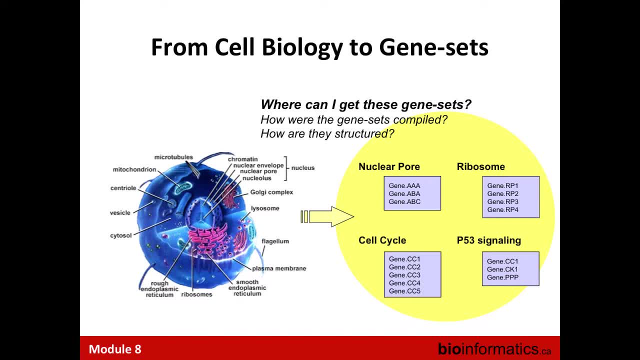 Absolutely That is. one of the major problems is the redundancy of various pathway lists, But these aren't pathways. Like gene sets are different from gene pathways. Yes, It depends on how you analyze them. The easiest way to do pathway enrichment analysis is to treat the pathway as a set pathway. 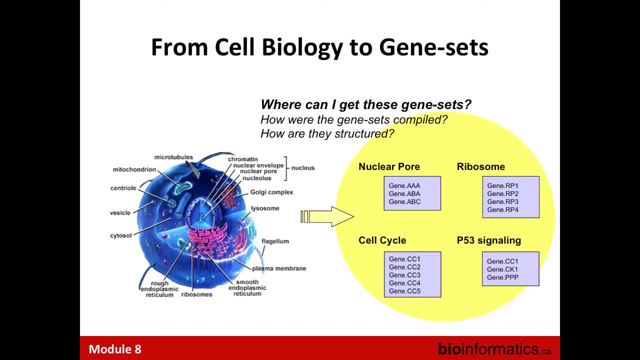 It's a set of genes without interactions. It does reflect the biology, right, It's not? It's the very simplest abstraction of biology. You add a layer of interactions. It becomes much more complex, much more meaningful, But you also reduce coverage. 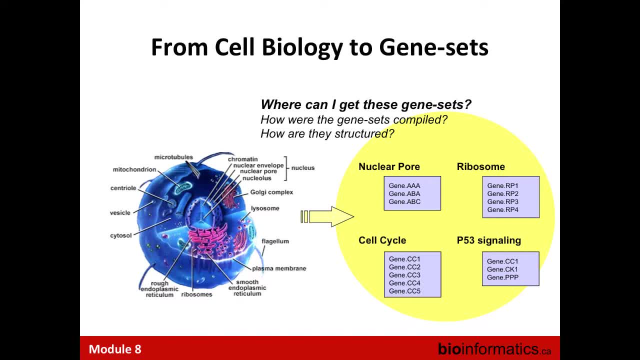 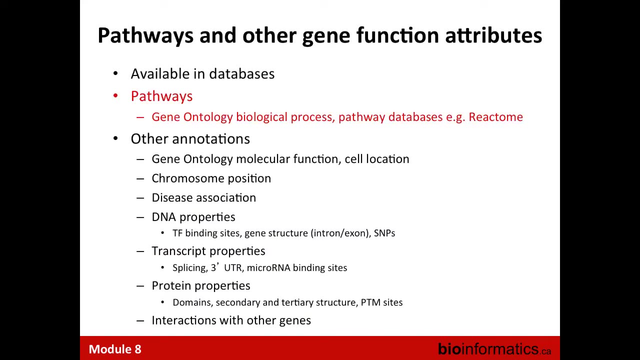 So not every pathway that we know of has very detailed interactions. What I'm saying is that a given gene can be involved in that, Absolutely Yes. More coming on that on the next slides. So what are pathways? I think everyone who works in biology or even in pathways will have a different interpretation. 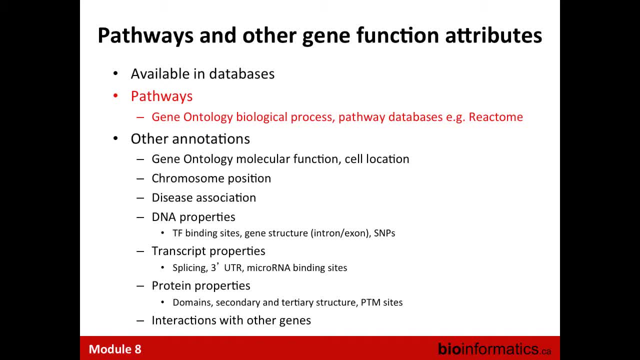 to what is a pathway In the context of this lecture, a pathway is mostly a set of genes that are working towards the same function in some way. They're ultimately coming from a database where human curators or curating algorithms have accumulated that knowledge over time. 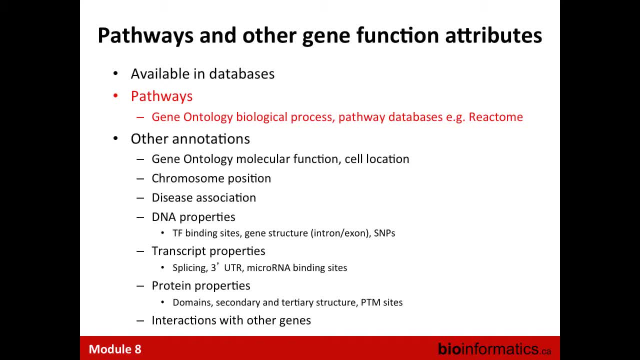 One of those databases is called the gene ontology. The gene ontology contains biological process, a particular structure that has thousands of sets of genes that have been associated to various pathways and processes. Other pathway databases include the Reactome developed here at the OICR, which generally 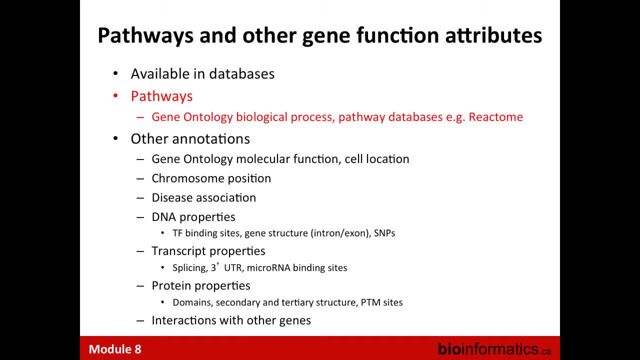 provides more detailed information also, including interactions and post-translational modifications, various details that we need to know how genes interact in order to carry out function. But if you have a set of genes, then the pathway enrichment analysis starts to look like a hammer with a bunch of nails. 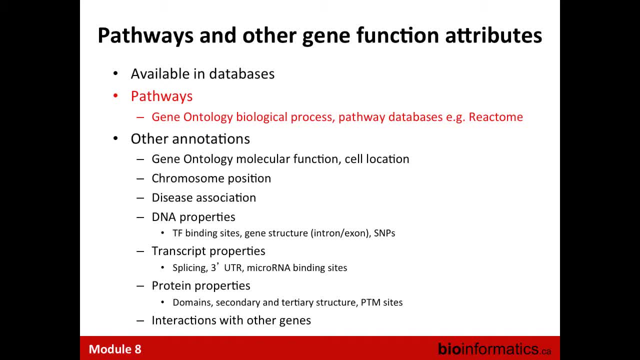 So you can use that type of an approach to do many other things. Besides these gene ontology biological processes. you can also look at cell components, hypotheses that maybe many of your genes that you detected are more enriched or present in a particular cellular component. 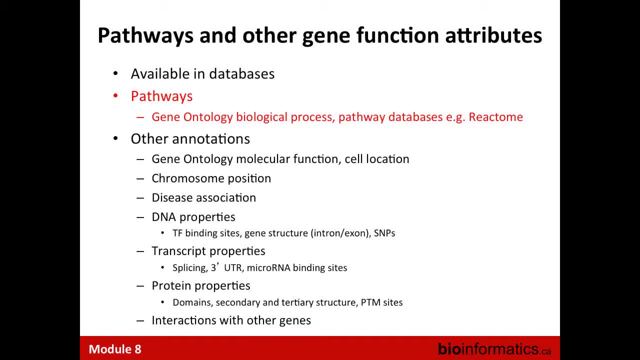 Maybe that has something to do with your experiment. You can look for disease annotations or positions within a chromosome, or perhaps transcription factor binding sites that all seem to be near your genes of interest. So the statistical framework is relevant and applicable to much more than just sets of 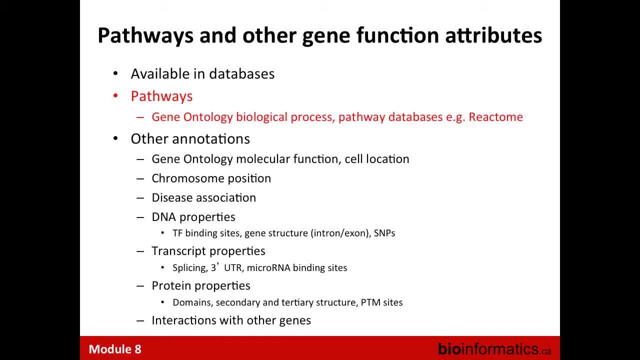 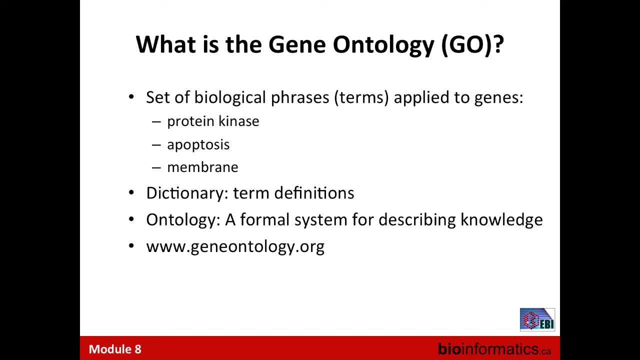 genes associated to pathways. So what is the gene ontology? This is the major resource that you are likely to use when you do pathway enrichment analysis, in the sense of testing gene sets. Gene ontology generally contains two things. First of all, it's a very complex and detailed dictionary of biological phenomena. 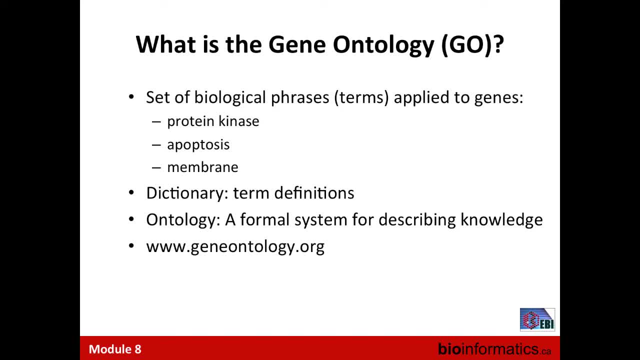 It's a set of words and concepts and phrases from biology and they are connected into this hierarchical structure. On the top of the hierarchical structure you may have something like the biological process, which is further distinguished into cellular processes and extracellular processes and so on, all the way to the very bottom-most levels of very detailed processes and functions. 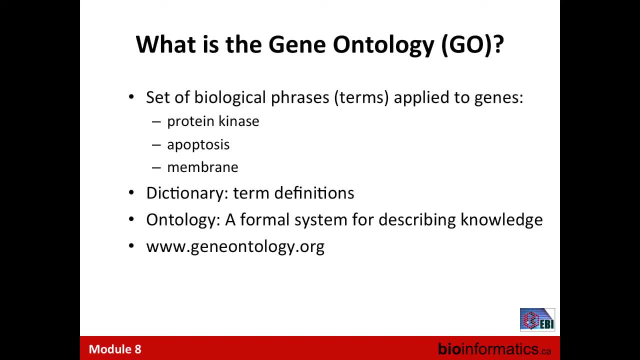 that maybe are associated to only one gene. So point one, the gene ontology is a dictionary, And the second part is that it's a set of annotations. So for many genes that we know of we have a set of annotations. We have little arrows that connect to these particular words in the dictionary or in. 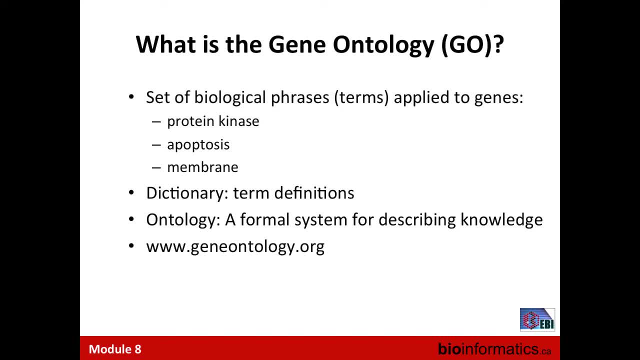 other words, we have found that that gene is associated to a particular process in the gene ontology, And gene ontology is general, so it applies to the biology of prokaryotes and deukaryotes and humans and mammals and fish and everyone alive should essentially be able to be mapped. 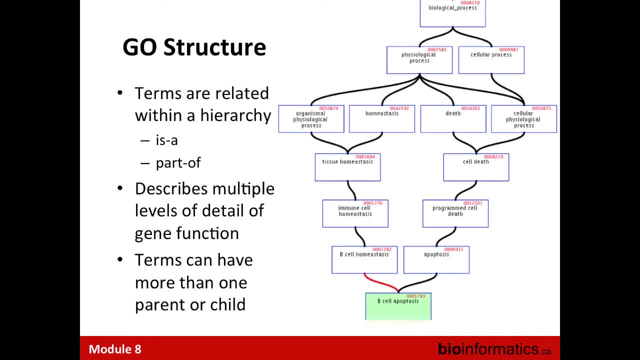 to the gene ontology. So here's actually an example of the structure that I described earlier. This is a directed acyclic graph or an ontology, where the terms are more general towards the top and more specific towards the bottom. They are connected through various logical relationships. 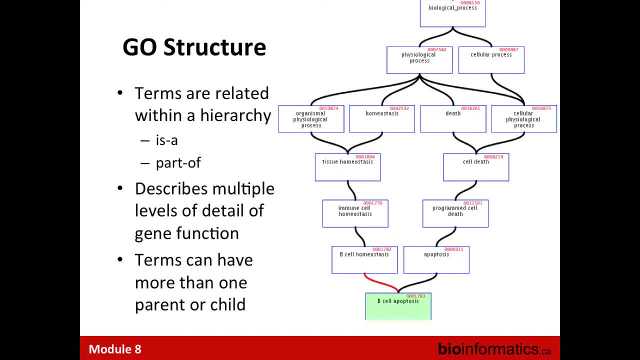 A biological process can be part of another biological process or it can be a more general or specific manifestation of it And these different terms, These terms describe multiple levels of detail of gene function and, as we already started to discuss, genes will be annotated to various levels of organization here and therefore. 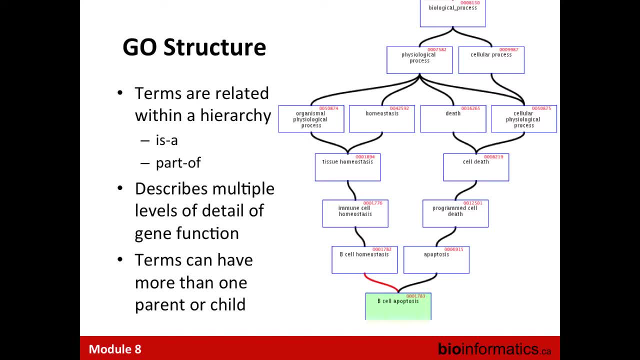 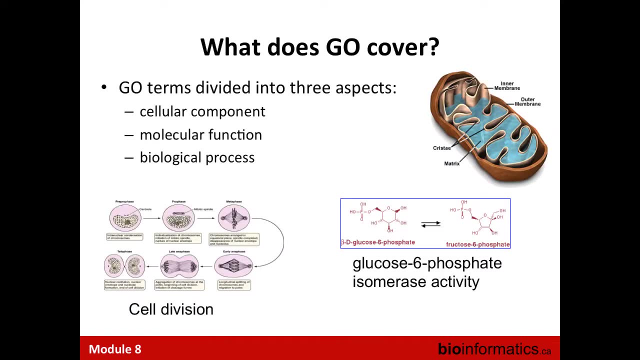 there's an immense level of redundancy, So one particular gene can be associated to hundreds or thousands of gene ontology terms, because these terms are interrelated each other through hierarchy. What does Go cover? Gene ontology has three different branches, So it looks like a tree upside down, and those major three branches represent cellular. 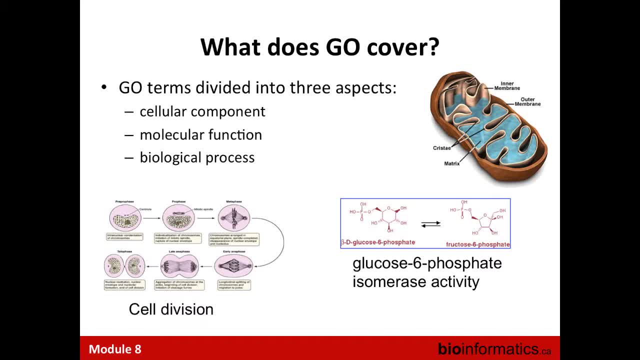 component, molecular function and biological process, whereas biological process is usually the most informative when you do pathway enrichment analysis. This is because this covers all the cancer-related processes, such as cell cycle proliferation differentiation. The molecular function tree is more towards biochemistry and cell components are what 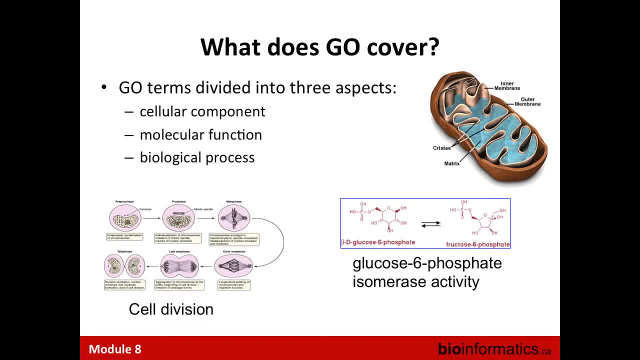 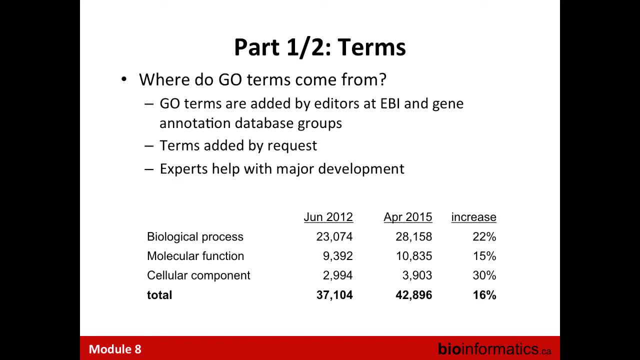 they are, So it's more difficult to interpret them directly in the context of cancer. Okay, so, as I discussed, there are the terms that make up the gene ontology and the annotations. Where do the terms come from? The terms generally come from two major sources. 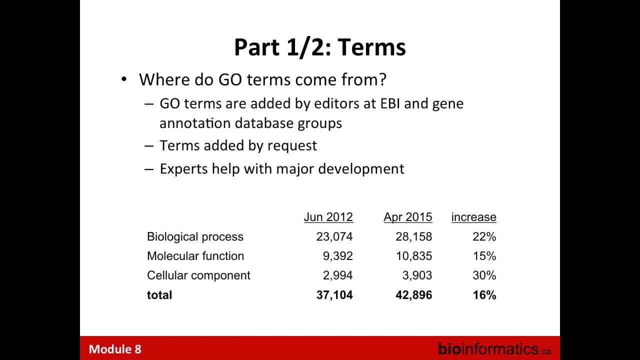 Literature curation is carried out by experts in the field- Gene ontology editors at the EBI in Cambridge- and also species-specific databases maintain their own gene ontology annotations, but they ultimately converge into a gene ontology database that is updated very frequently. I think it's updated every day. 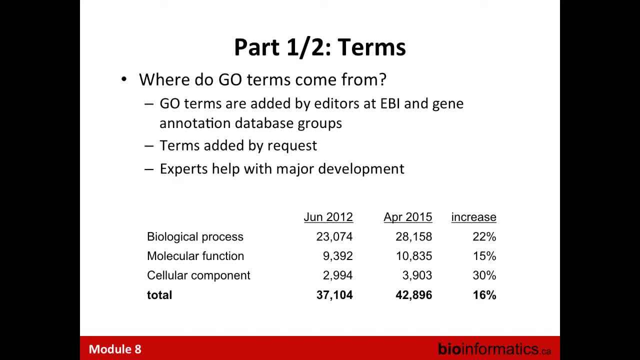 Terms are generally added by request and experts help with major development. because this is a live organism, so to say. It changes every once in a while and sometimes there are major changes like bigger branches being erased or created. And here are some numbers: 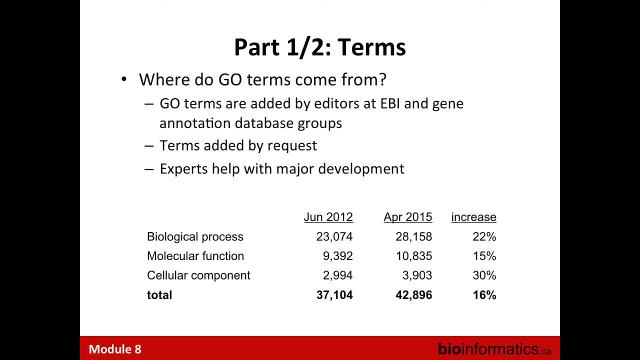 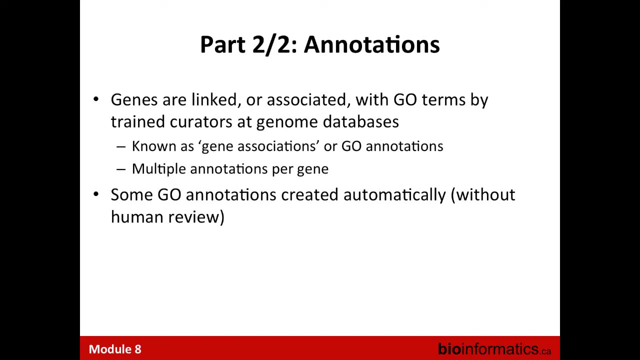 It's evolving actually pretty rapidly and it's worth paying attention to when you use an online tool to do gene ontology analysis- When was it last updated? Because that may actually change your results quite a bit. The second part of gene ontology are the annotations, and these are even more dynamic because people 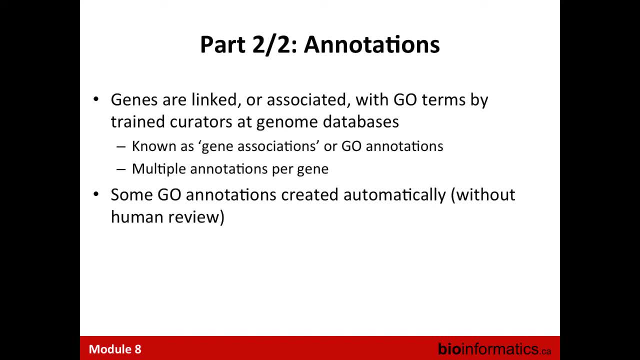 discover new gene functions all the time. Genes are linked or associated with GO terms by trained curations Or, more often, algorithms are associating these genes to various processes and pathways. These are known as gene associations or GO annotations and, as we already mentioned, 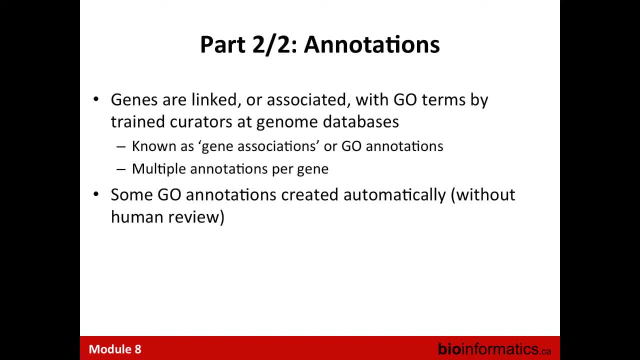 there are multiple annotations per gene. So why are there multiple annotations? One of them is that genes work in multiple pathways, obviously, But the other one is a more technical reason, because all of these pathways are hierarchically related. so are their gene contents. 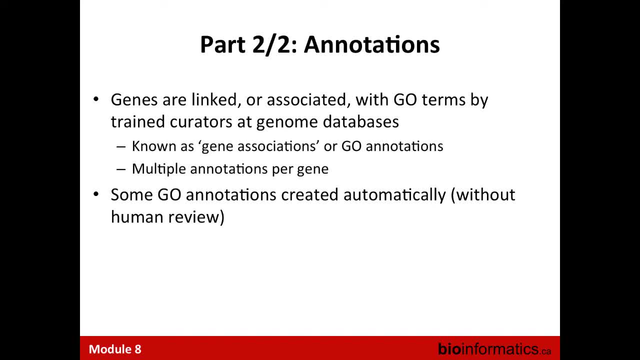 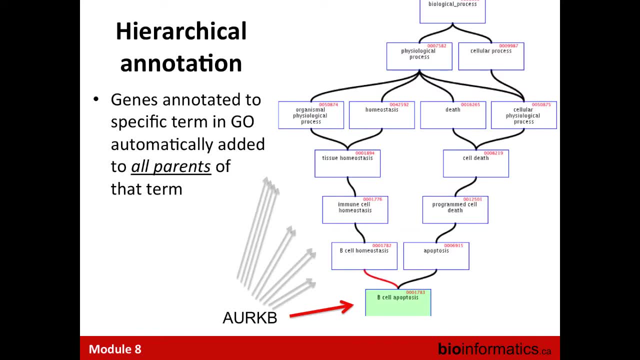 So if a particular gene is part of a pathway, it is also part of any parent pathways. So here's an example of the aurora kinase B, which is associated to B-cell apoptosis, a particular form of apoptosis. But in addition to that specific annotation to B-cell apoptosis, it is automatically also 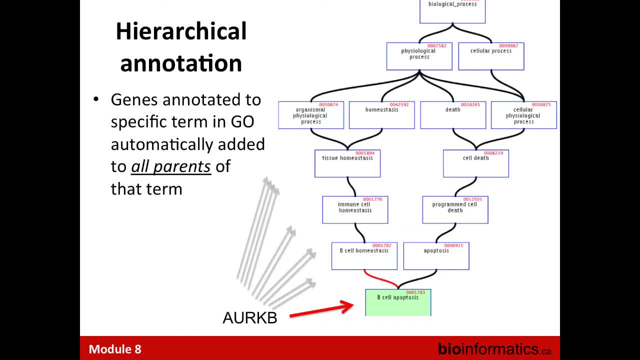 part of any other more general forms of apoptosis and cell death and so on. So if you look at this graph, you can see that it is all the way to the biological process. So you can see that by an expert curating aurora kinase B into one process or pathway. 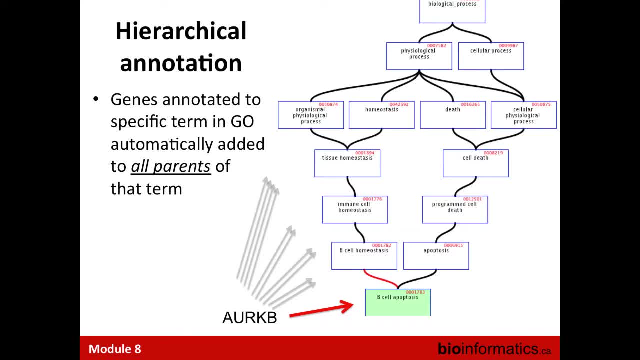 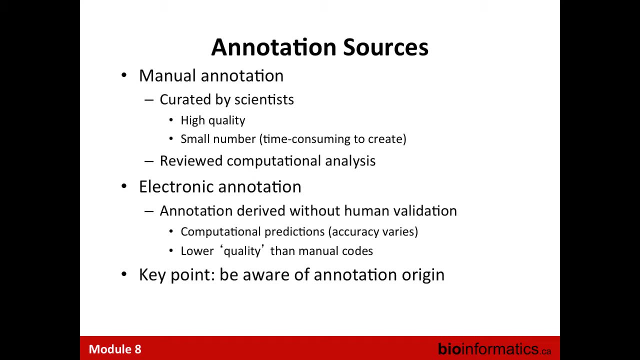 automatically. it gets replicated to dozens of other pathways that come above that particular pathway, So that creates a lot of information to crunch through. the algorithms or visualize Annotations come in different flavors. It also determines what is their quality in terms of scientific knowledge behind it. 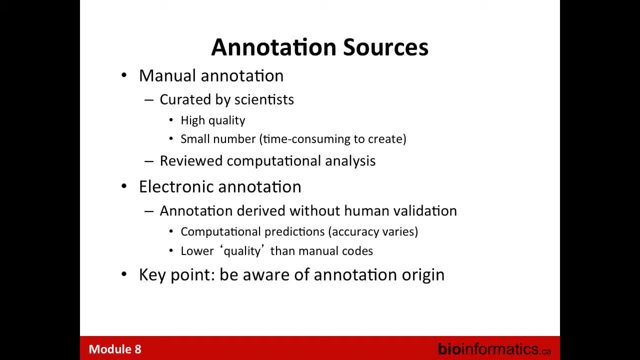 The most foolproof is manual annotation curated by scientists. It is generally high quality, but it's also a much smaller number of the total number of annotations, So only so many annotations can be curated by experts, especially these days when there are many high-throughput experiments, endless supplementary tables of genes associated to 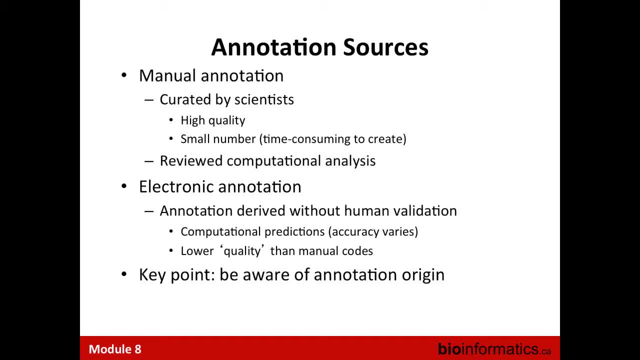 who knows what. And then many times these are the automated procedures that go through the different supplementary tables and associate the genes to the functions. So this is called electronic O-annotations. They actually make up the majority of annotations And in some tools that you use you have the opportunity to exclude electronic annotations. 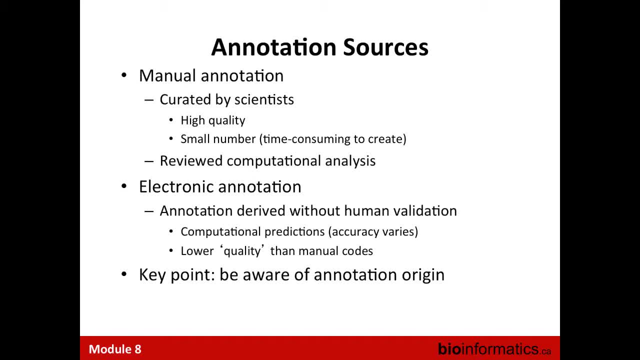 and only to stick with the more high-confidence annotations when you perform your analysis. So the key point is, once you find your favorite genes or favorite annotations, make sure to go back into the original annotations, or at least the quality scores of those annotations, and see what type of evidence was actually provided in order to make the conclusion that. 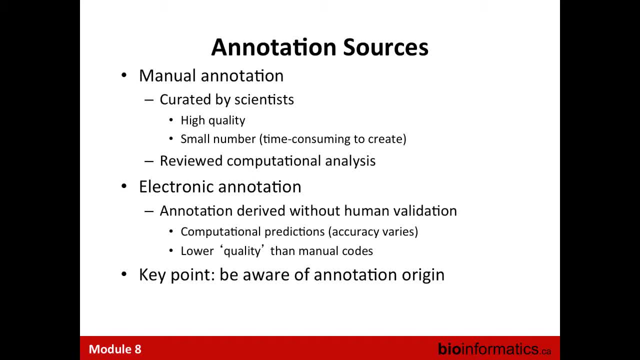 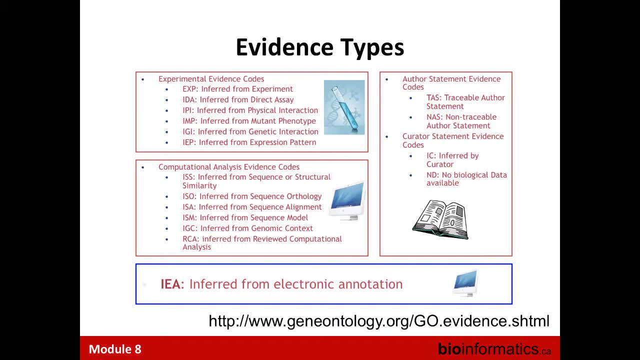 one gene is associated to another process. Some evidence types have been formalized, And you can see here that they range all from like a direct mutation experiment to gene conservation, to gene expression similarity, all the way to things like author statement or unknown, or electronic annotation. 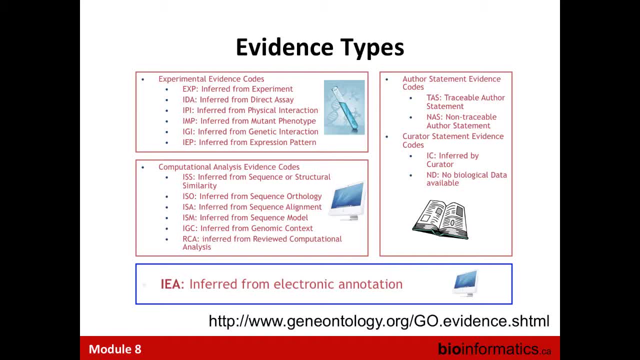 So that just tells you that certain results you should take with more salt than other results, And there are certain visualizations, including in the G-profiler software, that will allow you to have a quick glance of what type of evidence basically supports your findings. 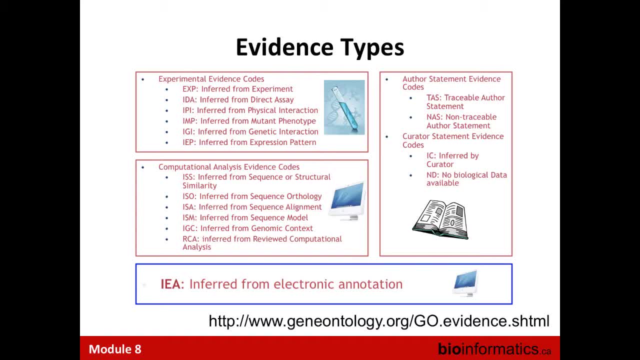 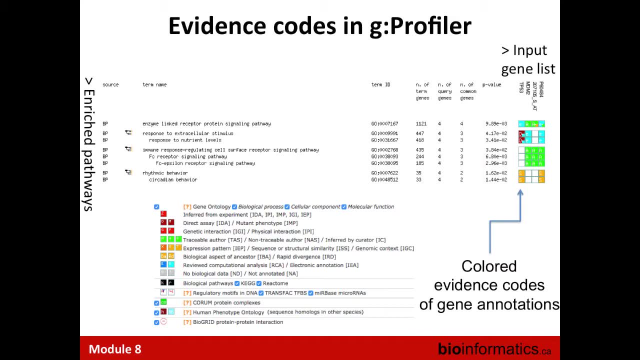 in terms of pathways and networks. Here's an example. There are various types of evidence. The types of evidence that support the relationship between a gene and the pathway are color-coded, So the darker, redder colors represent the high-confident experiments. 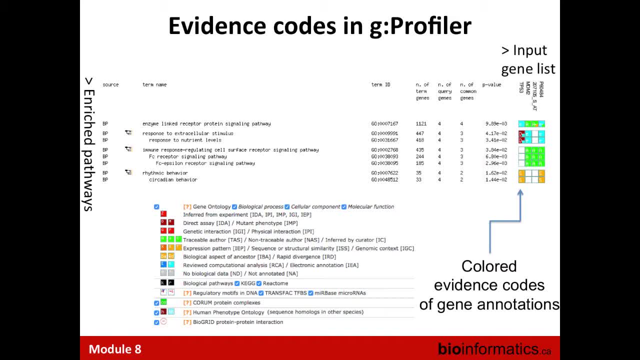 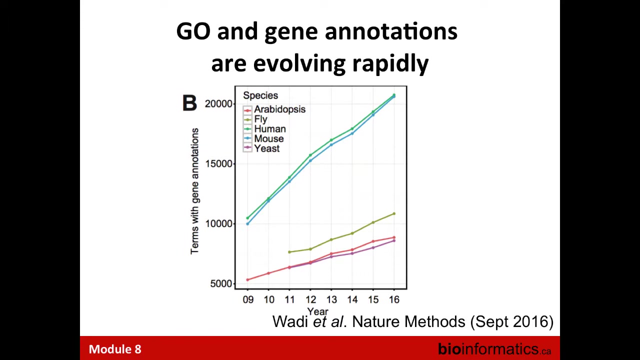 And then the lighter and bluer it goes, the more likely the evidence is high-throughput, maybe curated by an algorithm rather than a person, And that will tell you how confident that finding is in general, in context of known information. I've mentioned this a couple of times now, but it's worth mentioning again. 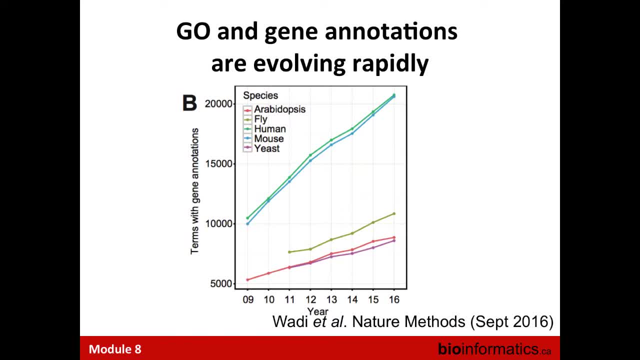 Gene ontology and especially the gene annotations are evolving very rapidly, So information gets past their best-before date quite quickly. This is a study that we performed in our lab here, where we went back into different releases of gene ontology and essentially counted how many terms there existed in the vocabulary at different years. 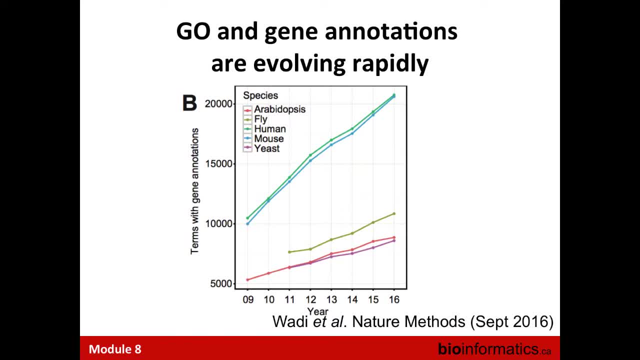 and how many gene annotations there existed in different years. In this figure you'll see that the number of terms or the thickness of the vocabulary of biomedical knowledge basically doubled over the past seven years, from 10,000 to 20,000 in mouse and human. 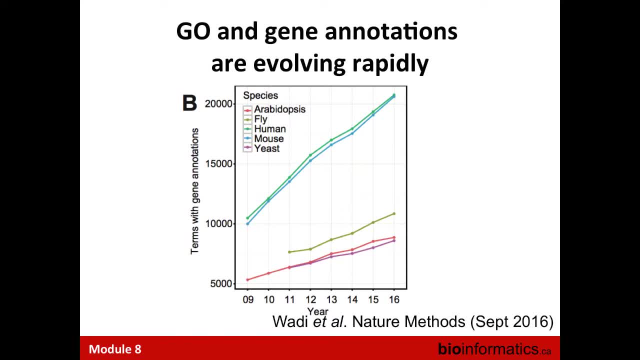 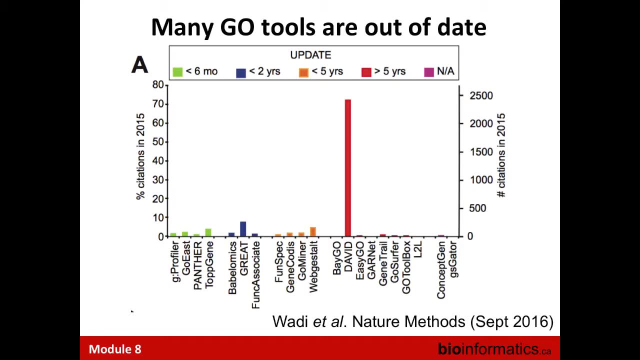 and other species showed similar growth. But where it really matters is when people do analyze their data using public resources, Because it turned out that many of the online web-based tools that carry out gene ontology analysis hadn't been updated for years, So we went out to investigate. how does that affect the results? 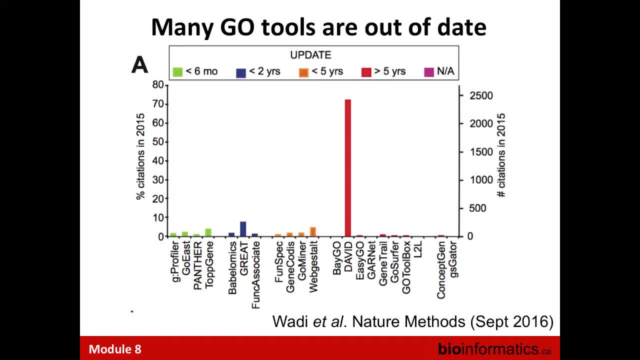 So it turns out that there's an elephant in the room denoted by this red big bar. The height of the bar shows the number of citations of that particular software in 2015,, so two years ago, It seems that it captured the majority of citations in the pathway analysis space. 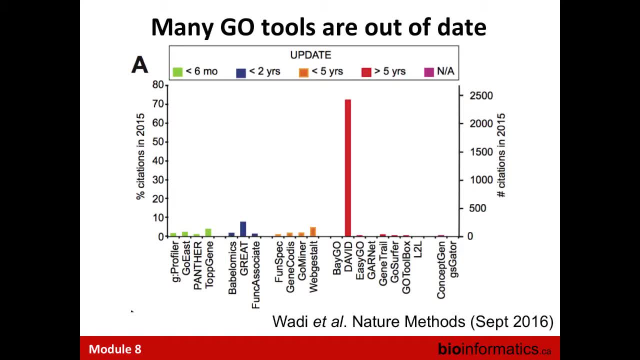 yet their annotations were more than six years old at that point. So that means that a lot of the knowledge from that tool that went into scientific literature is likely a little bit out of date or at worst it's invalid, And we sort of looked into that more comprehensively. 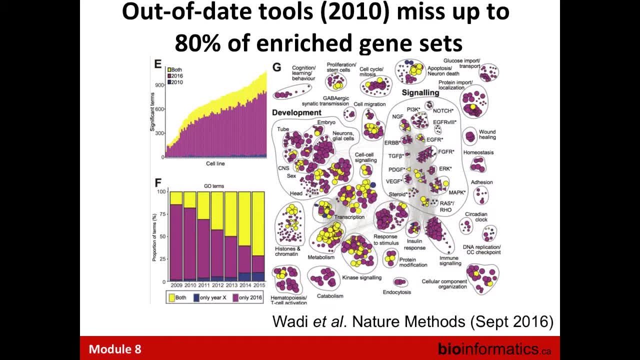 by analyzing the list of cancer driver genes from a brain cancer, just to compare. what does it mean? that one study would have used annotations from five years ago and another study would have used very recent annotations. And then this network visualization shows in purple the information that you get from up-to-date pathway analysis. 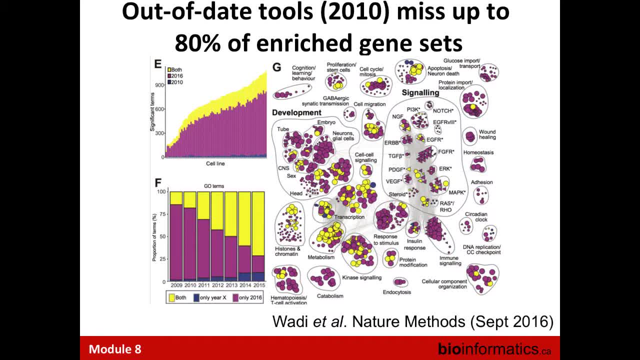 and the yellow shows you the information that you would get from both the updated version and the out-of-date version. So that's about four or five times more information that you would get when you use an up-to-date database, compared to a popular yet outdated database. 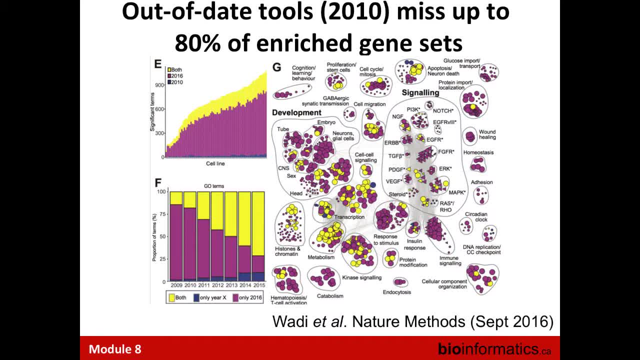 And in terms of cancer biology, this pathway analysis revealed some pathways that are now in clinical trials for cancer drugs that weren't obviously apparent in the earlier days, because these pathway targets haven't been discovered yet. So, whatever you do when you do a pathway enrichment analysis, 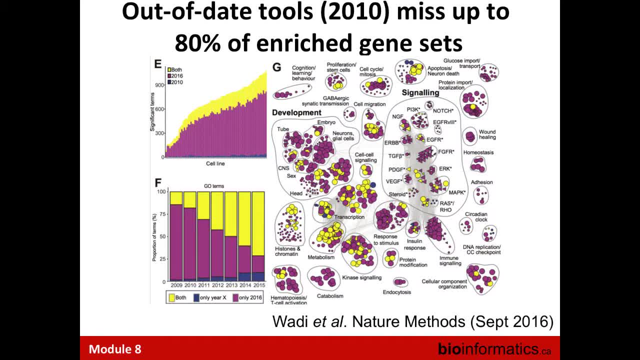 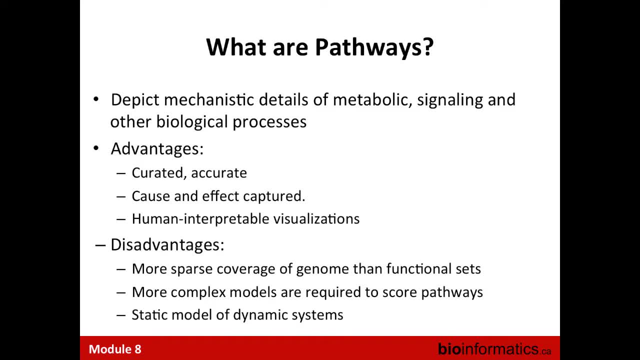 it's worth paying attention to when the information was last updated. No, it was updated after the bioarchive went viral, So it's fair to say that David has been updated, but you could speculate that some of that happened before because people noticed that it's really out-of-date. 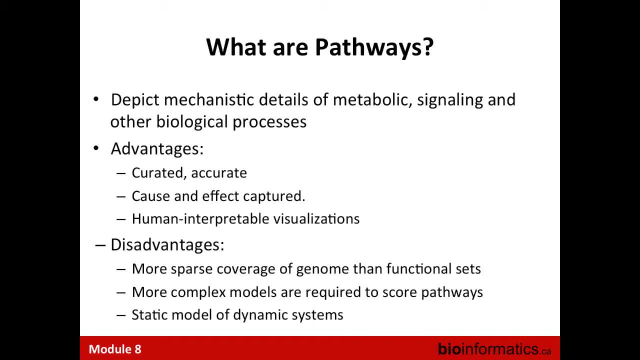 No, because everybody knows that they will keep coming back to that. So is there any good solution to that? They probably just run out of funding or something. Yeah, Well, they need to update it just consistently. No, but that's a good point though. 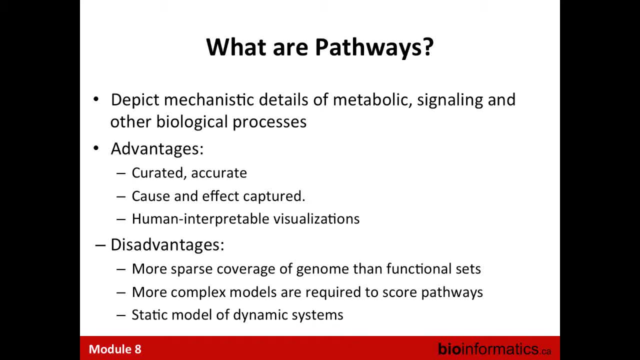 There are very few funding sources for maintenance and updating of databases. That's definitely a problem. Somebody should address that. Okay, so what are pathways? Everyone will have their own idea. Pathways are simplifications of molecular biology, where we attempt to depict the mechanistic details of various systems. 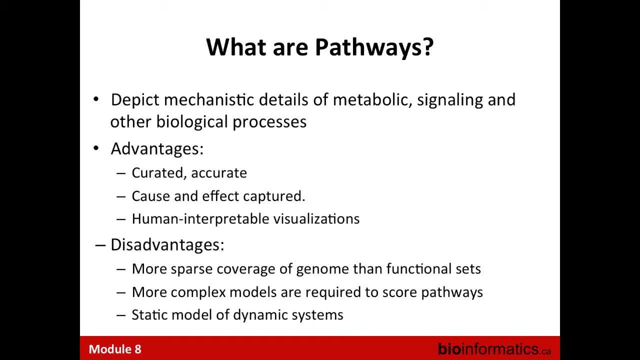 metabolic systems, signaling systems, other systems, Pathways are accurate to the level of detail that we know They're curated by humans. We try to capture cause and effect, and perhaps the most powerful way is to visualize these different relationships in a human-interpretable way. 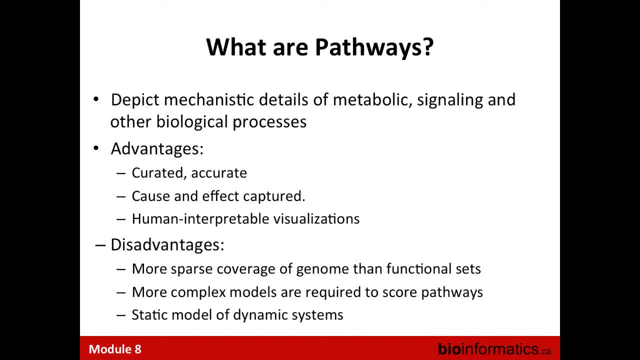 However, pathways are more sparsely covering the genome than functional sets, so it's easy to pile genes into sets, saying that someone, somewhere, found that these genes are all working on the same function. However, to define the relationships of various kinds of molecular interactions, 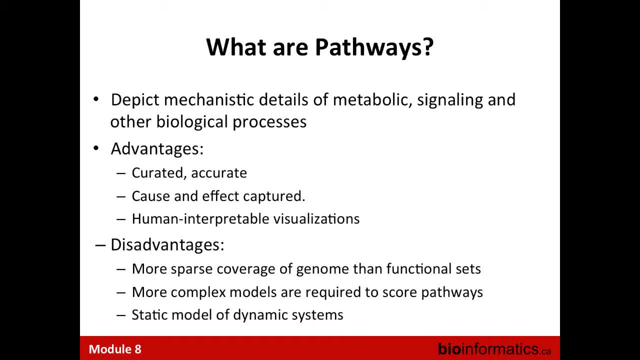 it's way more difficult And also, once you have a pathway that's laid out as an interaction diagram, you need more complex statistical and mathematical ways of interpreting that data in order to say something about, say, the prevalence of cancer. mutations And pathways could be static models or they could also be dynamic models. 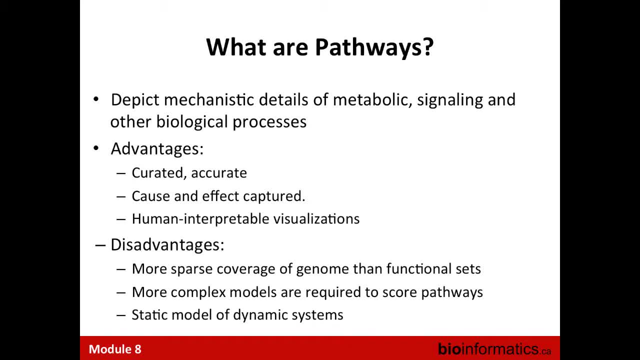 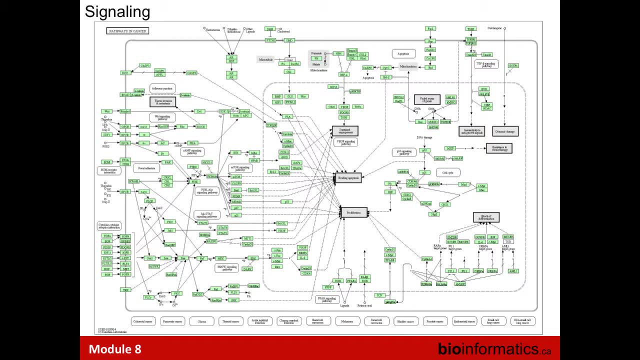 but in order to build dynamic models, we really need good, high-resolution data. So here's a small example. This is a small example of a signaling pathway from the Keck database. You'll see that it's immensely complex to understand and, given a set of mutations, 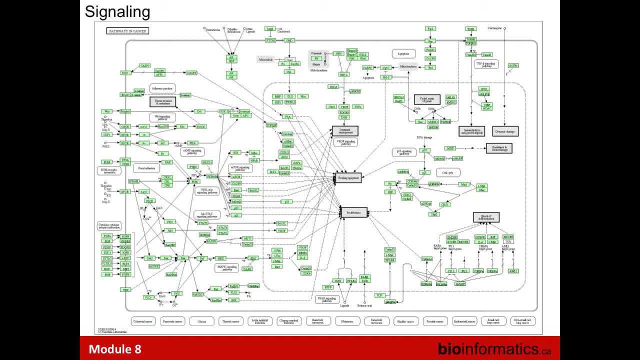 you could start to figure out what the mutation upstream is doing to the effect of downstream genes perhaps. but you really need good molecular data to perhaps measure that. So in the same samples you'd like to measure maybe protein levels and mutations and RNA levels and all these other things. 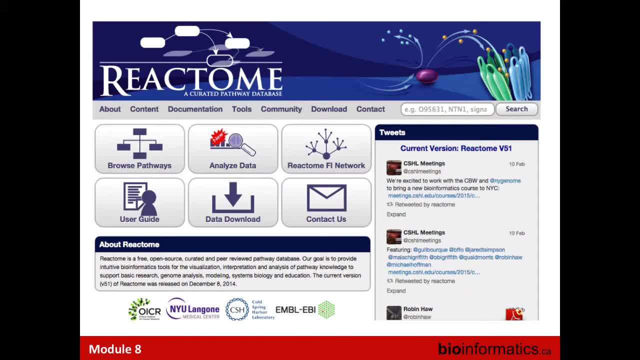 that you often don't have access to. A good resource for these pathway diagrams and toolkit molecular interactions is the Reactome database, which also provides several analytical tools to understand the statistical significance of your findings, and these will be discussed tomorrow morning in another lecture. 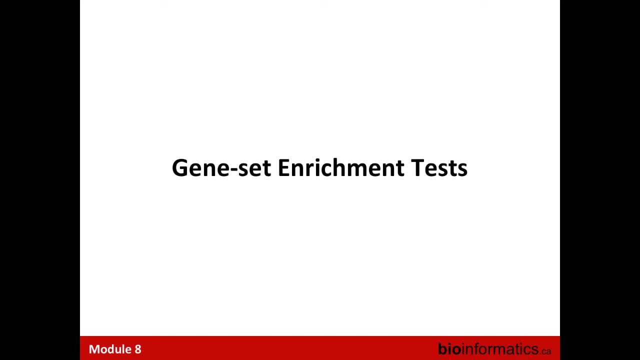 But here we are discussing the most simple types of tests, the gene set enrichment tests, which really describe your pathway as a set of genes, and they also describe your experimental list of genes and the goal is to find whether pathway genes are more present in your experimental results. 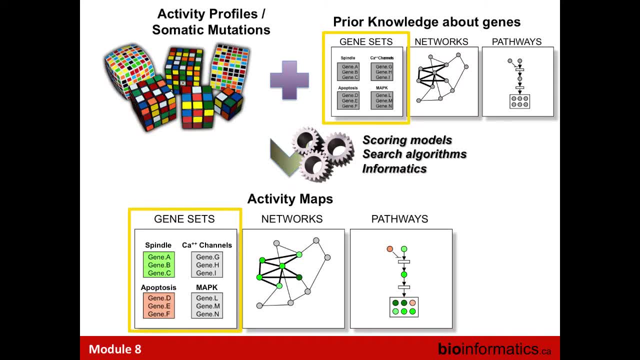 than compared to random chance- So I already showed you that figure earlier- where, on the one hand, we have some activity profiles, perhaps somatic mutation from cancer genomes, and we have prior knowledge about gene sets, genes that are involved in various processes or pathways. 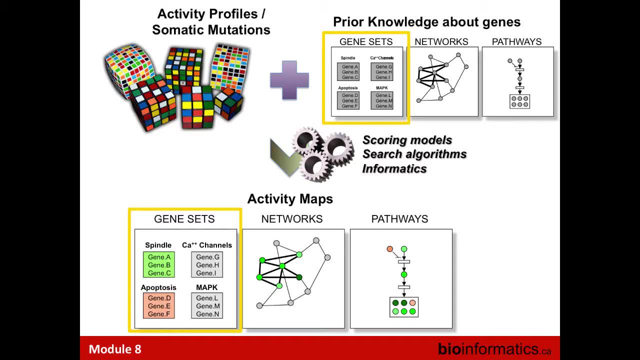 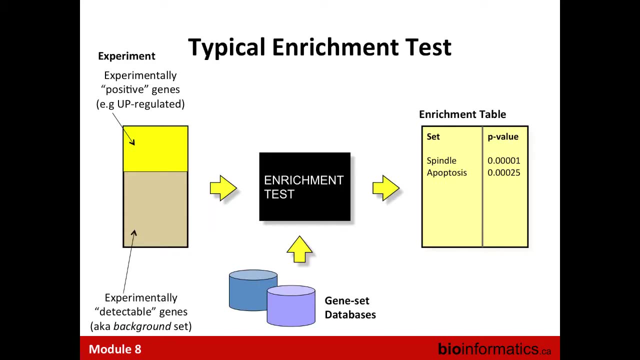 And using statistics we can determine which of those prior knowledge-related gene sets are actually overrepresented among our molecular information, so activity profiles or somatic mutations or gene expression values or so on. So a typical enrichment test looks like this: On the left in yellow, 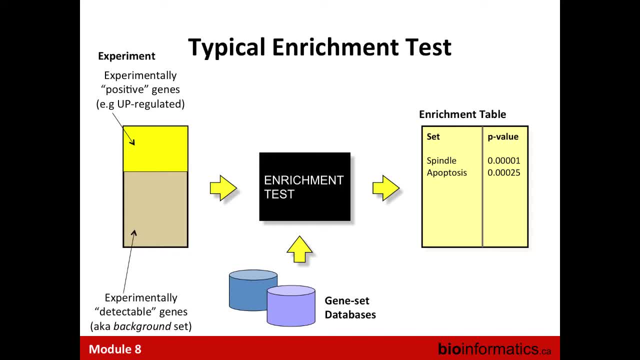 you'll see your experiments that experimentally derived positive genes. So these may be genes that, for example, had a detectable amount of positive selection in your cancer genomes. They had more than expected number of mutations. And then the bigger box in tan and yellow. 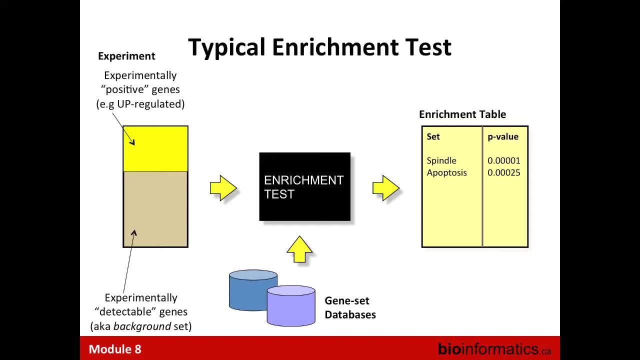 represents all the genes that you analyzed, So perhaps you were looking only at the protein coding segment of the genome. You looked at 20,000 genes. Out of those, 100 showed more than expected number of mutations. This defines your background and foreground sets. 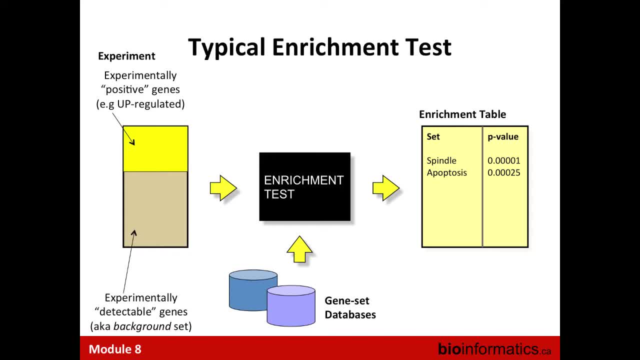 So these are all the genes that you studied. Now you have a black box called enrichment test which will, as additional input, take all the gene set databases as input. It will crunch through the different gene sets and decide that some of the gene sets 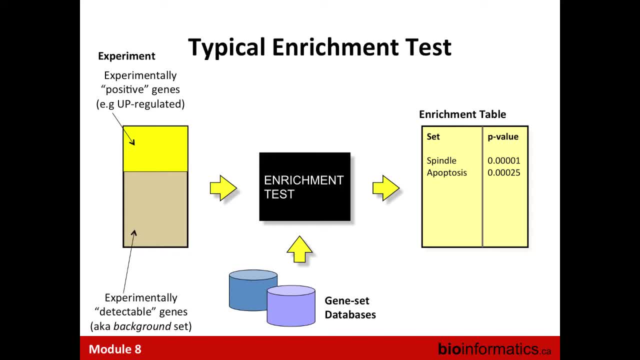 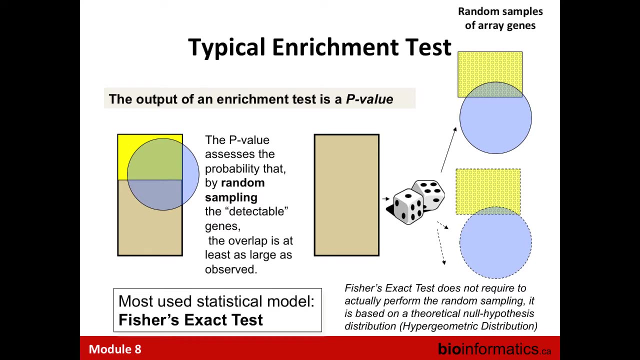 are particularly representative of your experimental data. So maybe spindle function and apoptosis were some of them, And they come with a statistically significant p-value. You report the p-value, visualize the results and publish. And so what does the p-value really do? 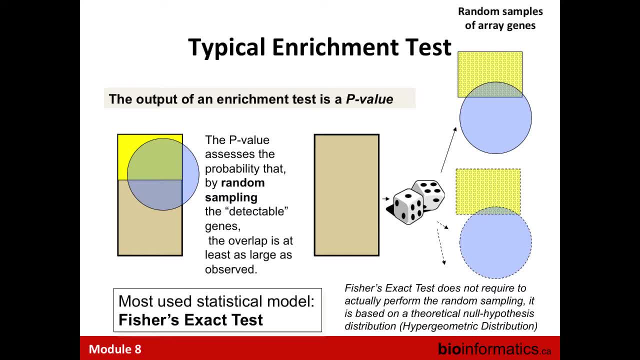 One of the more common p-values that we compute is a Fisher's exact p-value or a hypergeometric test p-value, And the p-value assesses the probability that by random sampling of genes from the detectable set of genes you'll get an overlap with a particular pathway. 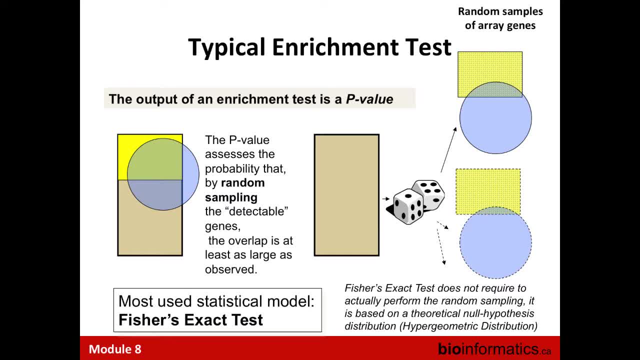 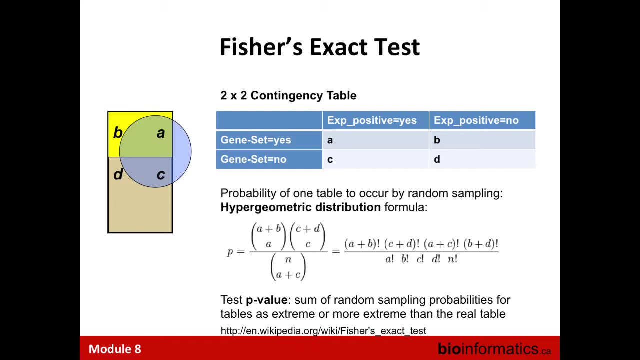 that is as large as the pathway that you observed To compute the Fisher's exact test. you essentially build a contingency table where you decide whether a gene set, whether any gene is present in a gene set, yes or no, or whether any gene is present. 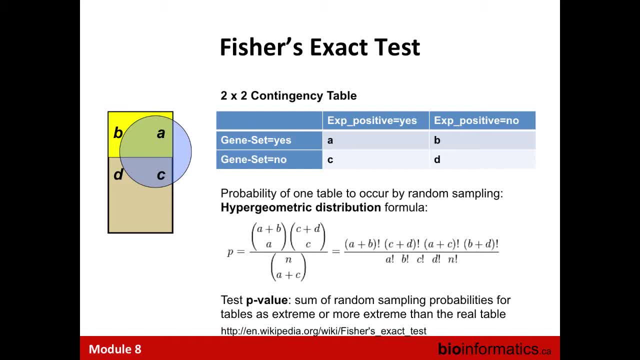 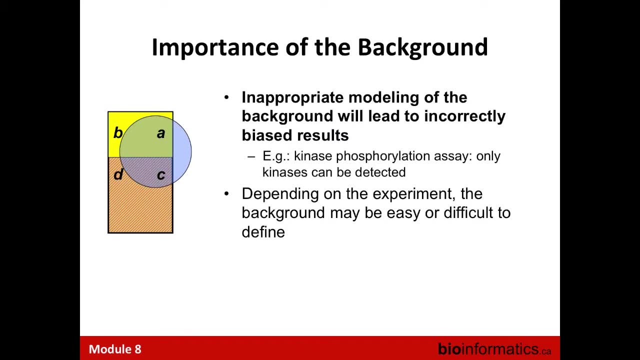 in your significantly mutated list of genes, yes or no, And you estimate the probability of seeing that by chance using the hypergeometric distribution And then, if the gene set is more overrepresented than you would expect, by chance you can report that that pathway? 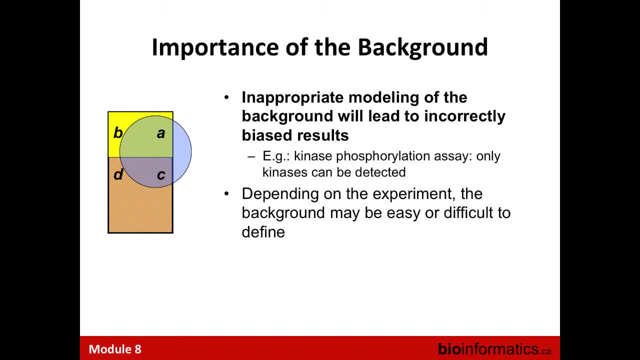 maybe has some sort of a significance in your experiment. Now, a really important thing to pay attention to is the background rate, So the experimentally detected genes is usually set to the entire set of protein-coding genes in any pathway tool, And that assumes that you are actually actively able. 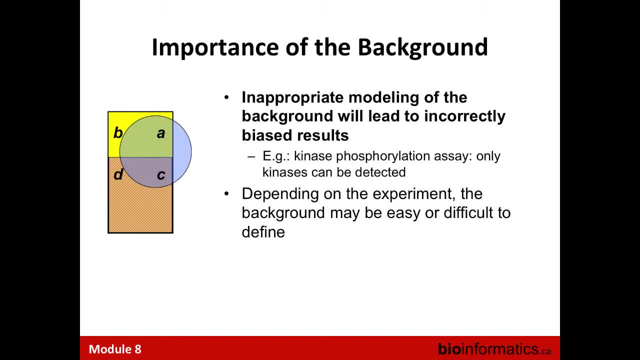 to measure any of the detectable genes in the genome. So perhaps this is the case in a standard sequencing study, where you were actually actively sequencing all the exons of all the genes. However, let's imagine a situation that you're looking at an older data set. 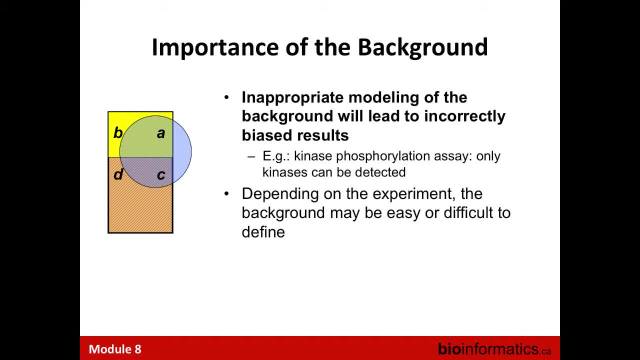 where only 100 genes were sequenced. So maybe that's part of a gene panel of very well-established cancer genes and any patient in that set only was sequenced for that 100.. So the rest of the almost 20,000 genes. 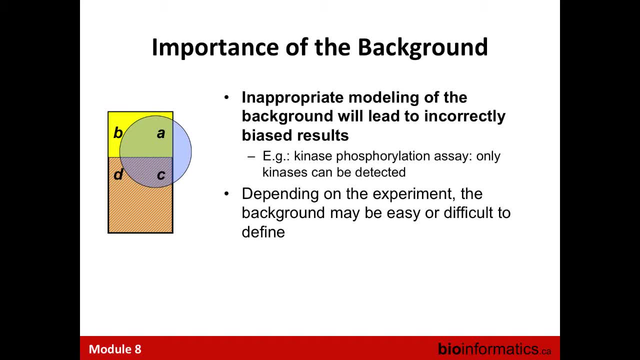 had no signal whatsoever. If you run your statistical enrichment test now using the entire set of coding genes, you will get very large inflations in any pathways because any gene that you come out with that has a meaningful score will only be sampled from that 100. 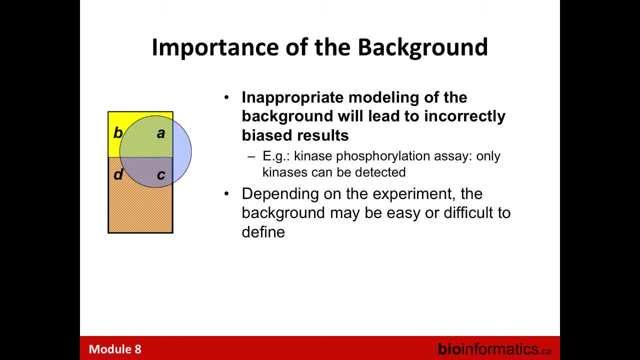 that comprise the original panel that you sequenced. Another example is that maybe you're doing a phosphoproteomic analysis and you're looking for the proteins that get phosphorylated under a particular cellular condition. However, it turns out that only about two-thirds of the proteins 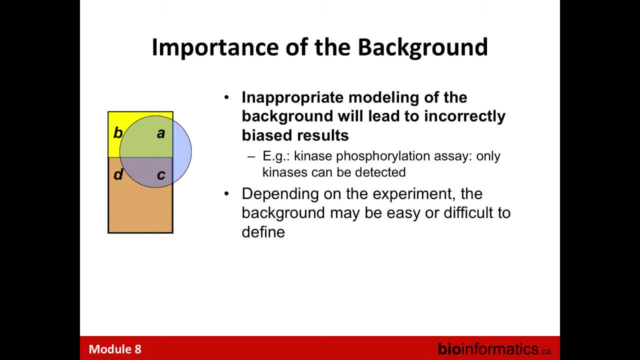 can get ever phosphorylated, and the other proteins are not phosphorylated at all. Therefore, if you do a pathway enrichment analysis that considers all the genes in the genome, then you will naturally get an enrichment for phosphoproteins, because these phosphoproteins are the ones 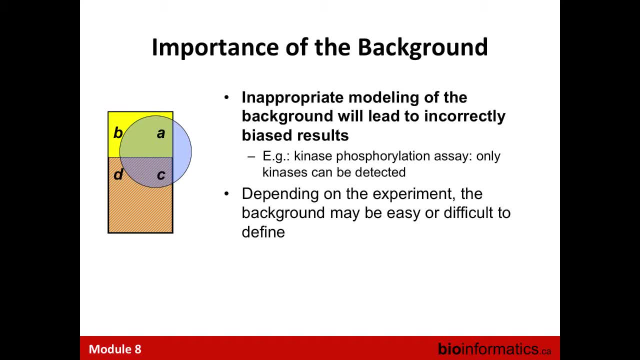 that ever get a signal because of your experimental design. So therefore, when you do a pathway enrichment analysis, think about this a little: Did all the genes in your genome get the signal according to experimental design? And if not, then you need to select. 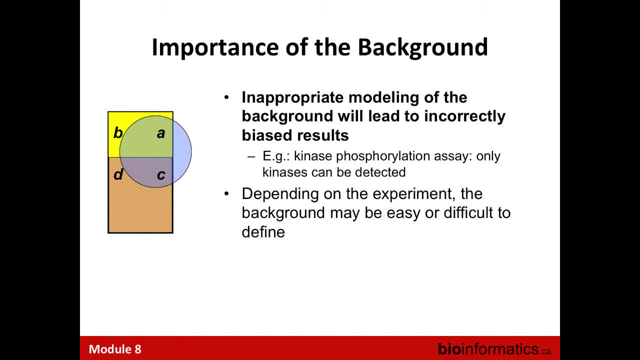 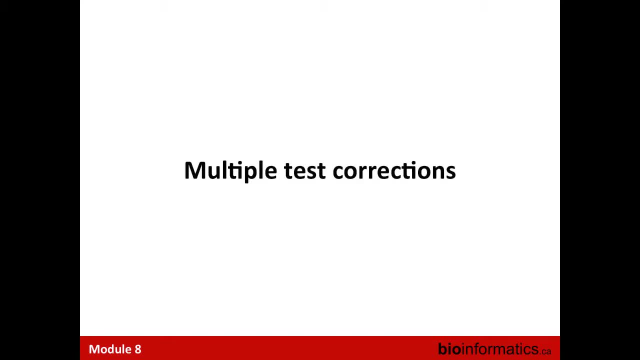 a more conservative pathway test where the background gene set is explicitly defined as the list of genes that were part of your experimental design. So, multiple testing corrections: I'm sure that many of you have heard of them and maybe actively use them. They are essential in the era of genomics. 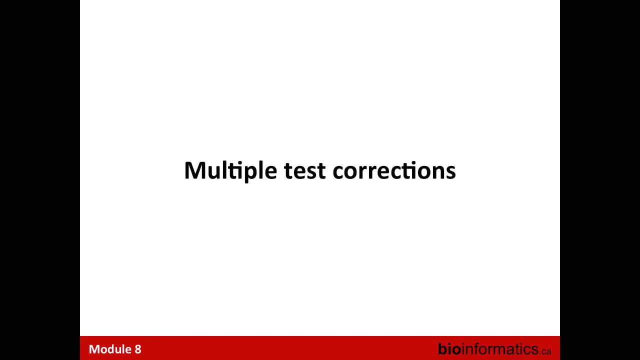 because we measure many things at the same time. We conduct hundreds of thousands of statistical tests and therefore it's very likely that one of those statistical tests will win the p-value lottery just by chance, and you'll get a very meaningful result that looks meaningful but can be noise. 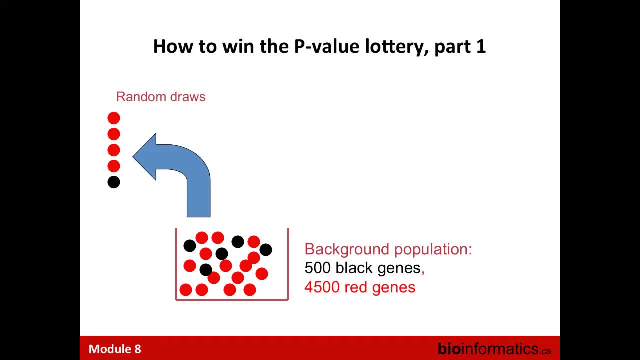 So here's a visualization of what this fission exact test actually looks like. Say, we have a bowl of genes or balls and most of them are boring genes, So they're red, and some of them are really interesting genes, say the cancer driver genes that are known. 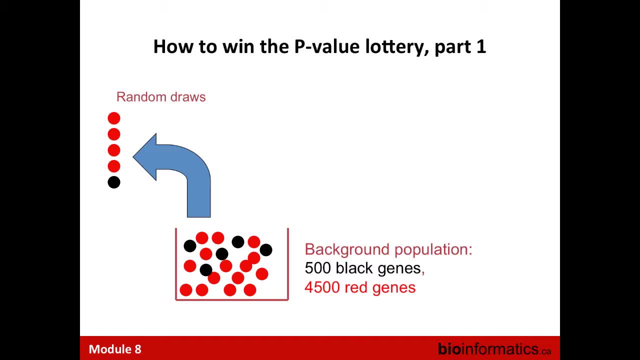 These are black. So if you just take one random draw then you're quite likely to get. so mostly sample the red balls and none of the black ones. But because in genomics we carry out thousands of tests, for example in the pathway enrichment analysis. 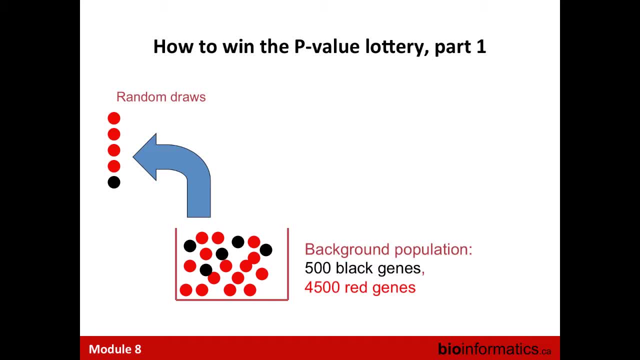 we can easily look at 10,000 gene ontology terms. then we sample, and sample, and sample and then ultimately, a few thousand draws later, we pull out the bowl a handful of balls or genes that are all really interesting, all the black ones. 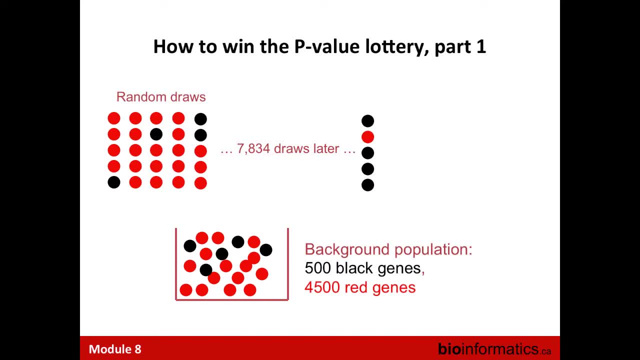 Because of that we need to apply multiple testing correction, So any p-value can be taken at face value, because if you conduct a series of them, it's more likely that at least some of the series will look really significant, even though there is no reason to see that. 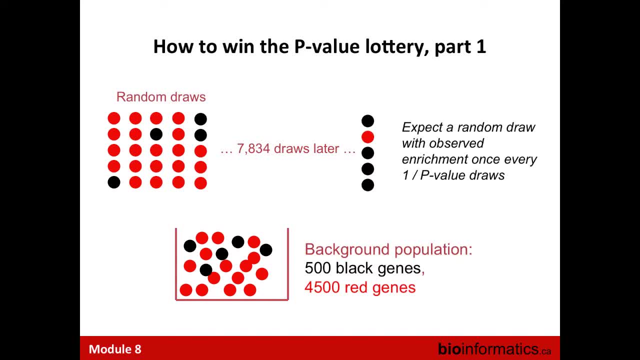 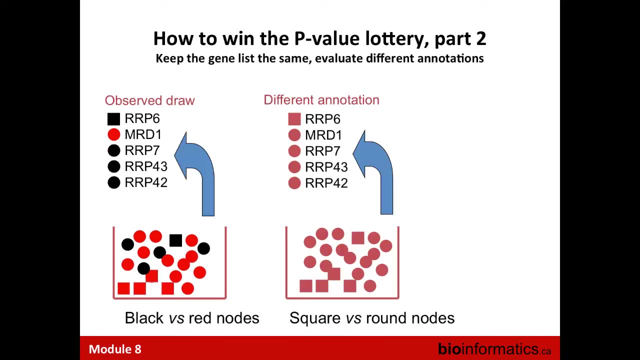 So in essence you can expect the random draw to have an observed enrichment once every one over p-value draws. So if you draw a good number of tests, then one of them will look very significant just by chance. Another way of doing it is not sampling the same ball. 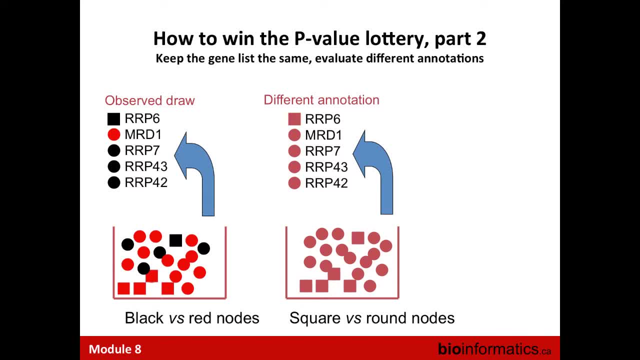 but sampling different balls every time. So one time you sample black versus red genes, other time you sample square versus round genes, other time you sample apoptosis genes versus schizophrenia genes. but if your experiment comprises a large number of those tests, you need to take more care to interpret the p-values. 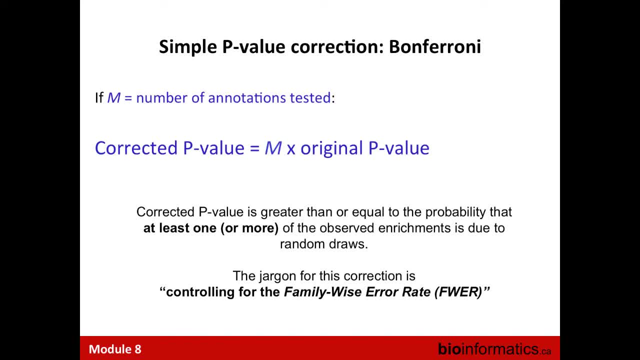 The simplest p-value correction is the one called the Ponferroni correction. This is very stringent and it's also a little out of date. so mostly for teaching purposes, If you have m tests and then each one of them provides a p-value. 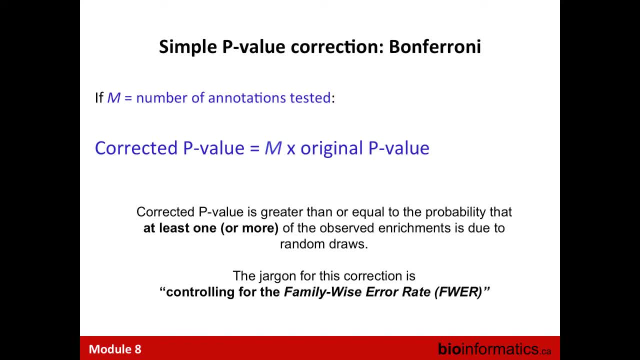 then you need to multiply each p-value by m, so say 100, to get the actual post-correction p-value. So this is very stringent. So suddenly your 0.001 becomes 0.1, and you can't report anything. 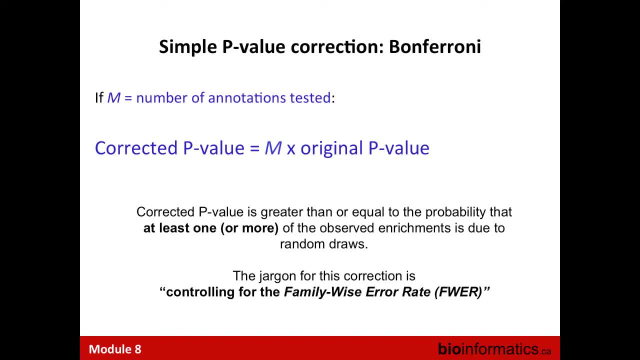 Now the assumptions of that test are also quite stringent. So you apply this correction and afterwards you are certain that there are no false positives. So the corrected p-value is greater than or equal to the probability that at least one or more of the observed enrichment 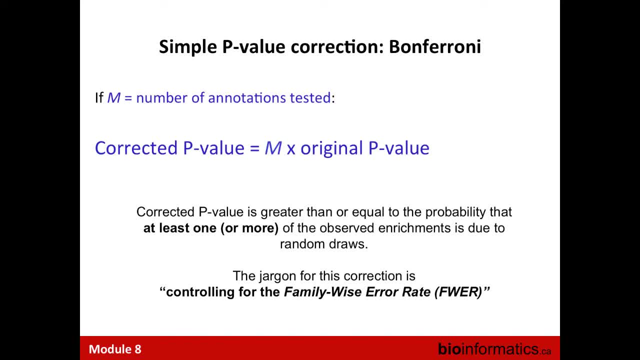 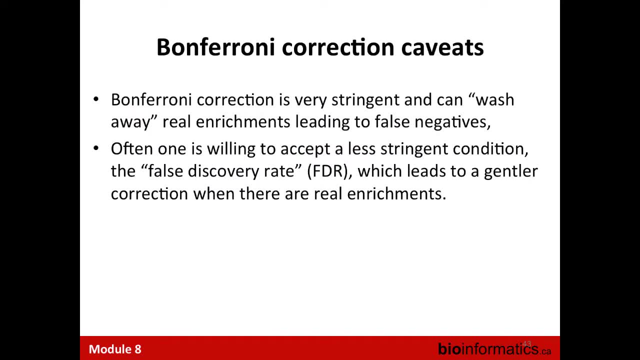 is due to random drops, so at least one, And you control for the family-wise error rate, which is a very stringent correction, So that we already discussed- You may have actually very nice-looking and valid results. but if you apply Ponferroni- 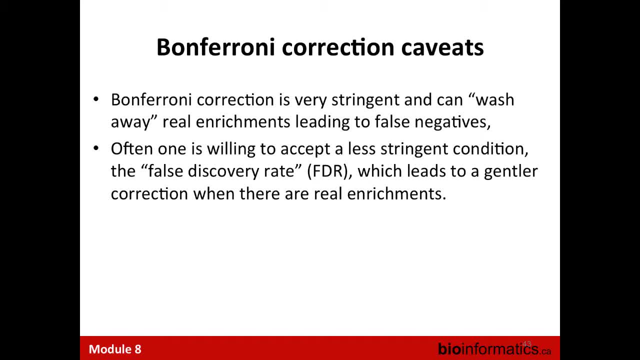 and you go through a large number of tests, then you are quite likely to wash out any important signal and just remain with no significant results. So therefore, often in genomic studies we are willing to accept something that is a little weaker, So we accept weaker results. 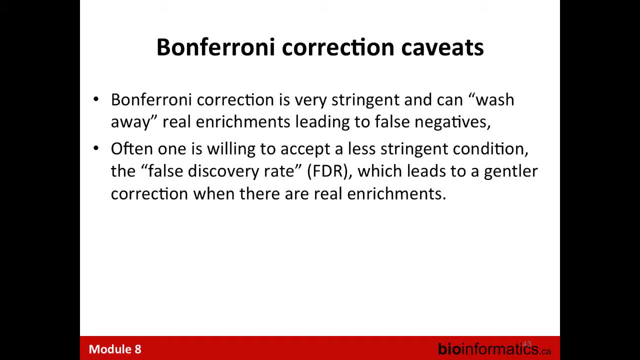 we accept more false positives among our results, but we actually gain results with that caveat in mind. So this is called false discovery rate or FTR. I'm sure that everyone has encountered that. FTR is the expected proportion of the observed enrichments. 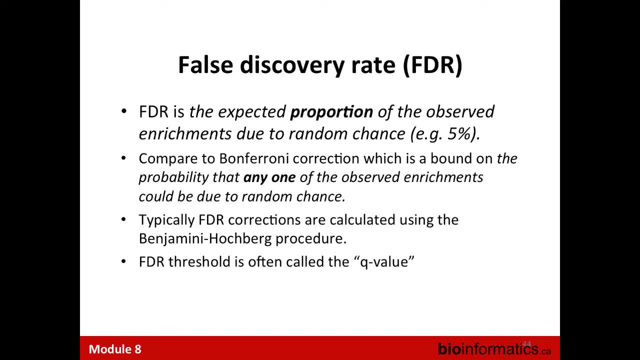 are due to random chance. So instead of putting a very focused count of one false positive or more, you say 5% of the results could be wrong. So if you have 100 results, maybe 5 of them will be wrong And typically the FTR correction is calculated. 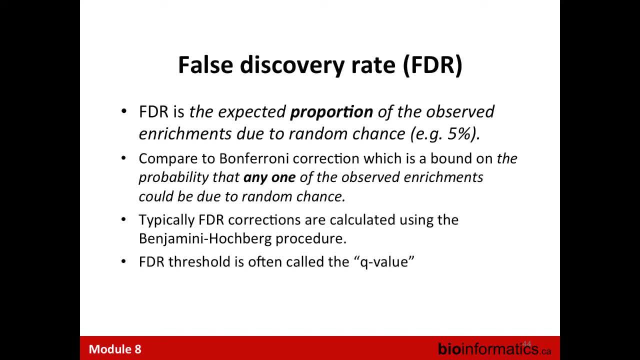 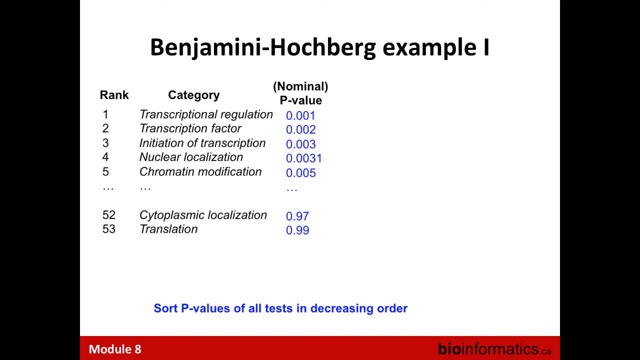 using the Benjamini-Hoppe procedure, which is state-of-the-art in genomics, but there are many variations of this procedure for various situations. Let's try to walk through an example. This is maybe a pathway enrichment analysis, where the nominal p-value coming out from a Fisher's exact test 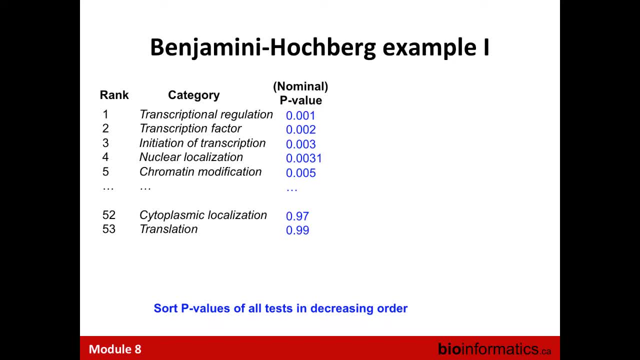 gives you the number of random cases that you would count to see that observation occur properly. So if you look at this graph, you can see that each p-value is multiplied by a random chance and you see that they're ranked by their significance, starting from 0.001 all the way to 0.99.. 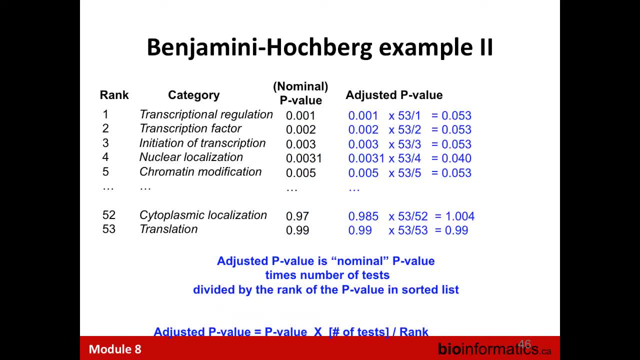 So the way the Benjamini-Hoppe correction works is the following: First, you multiply each p-value by the rank of it in its list, so you'll see that there were 53 of them altogether, for example. Then the first one is multiplied by 53 over 1,. 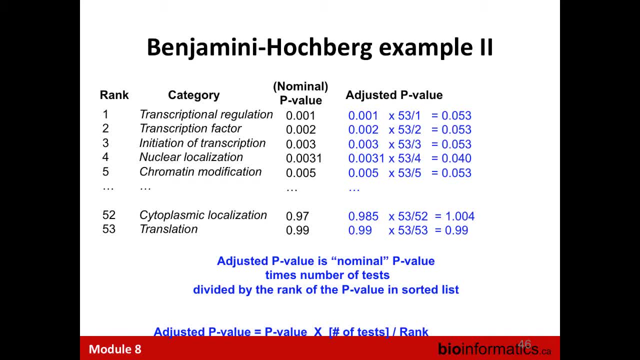 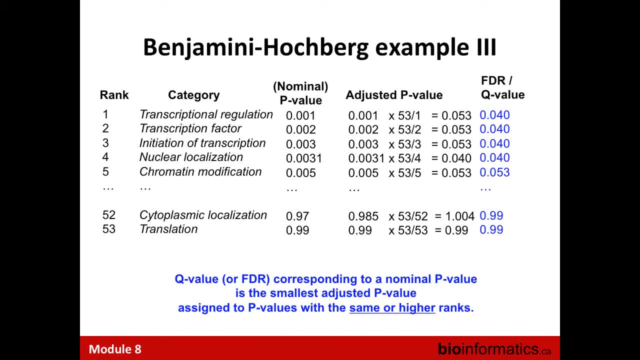 and so on. so they get adjusted, And then this is similar to the way adjustment happens in the Ponferroni. Now the Q-value, or the final post-correction p-value or FTR value is computed such that the corresponding. 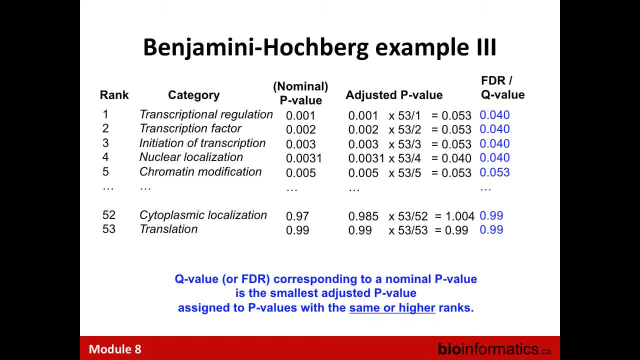 Oh, let me rephrase this: Corresponding to a nominal p-value is the smallest adjusted p-value assigned to p-values with the same or higher ranks. So it becomes like a staircase Instead of a flat series of values. the bottom-most value has this equal FTR value to the top-most value. 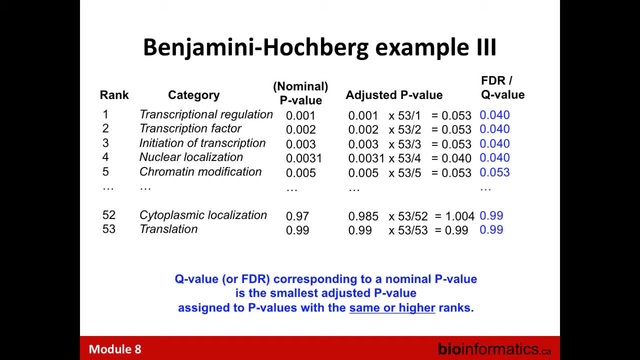 and further down, another set of pathways will have similar values all the way to down And now, based on that correction, you will filter the 5% threshold, seeing that the first four will become significant and the rest will be corrected. But the first column, where all of the visible pathways 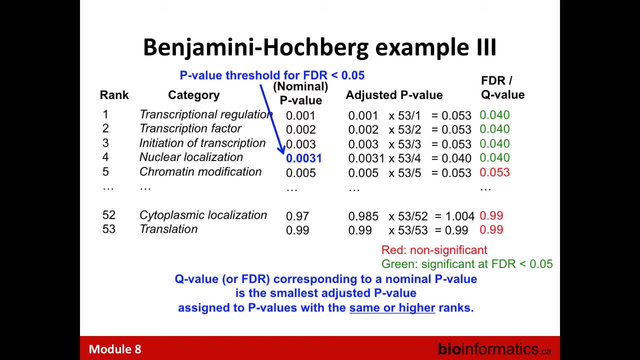 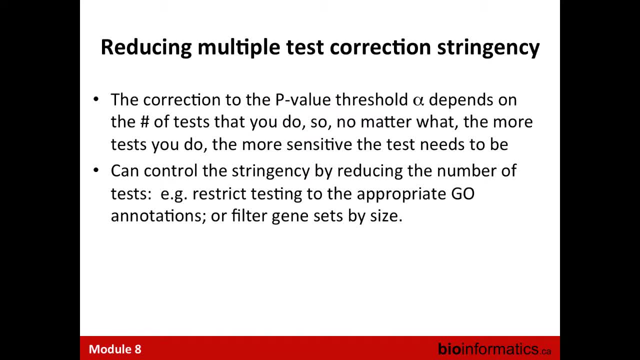 had a significant p-value. the corrected p-value is way more conservative. So, as you see, when you're really interested in getting out important or significant p-values, but you still run a large number of tests, you can't really get around it. 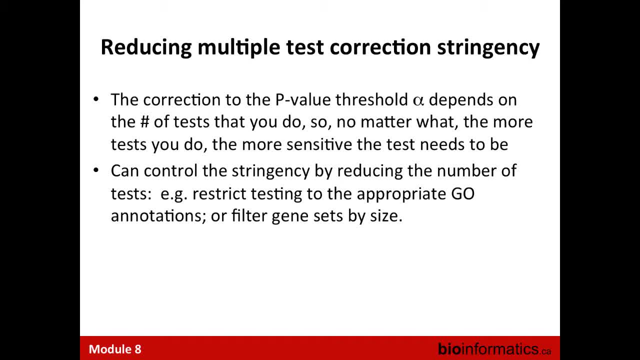 The more tests you run, the more conservative you have to be about each individual p-value. So one way to get around this is just to do a little less tests. You may want to look at your set of results that you're testing a little bit more carefully. 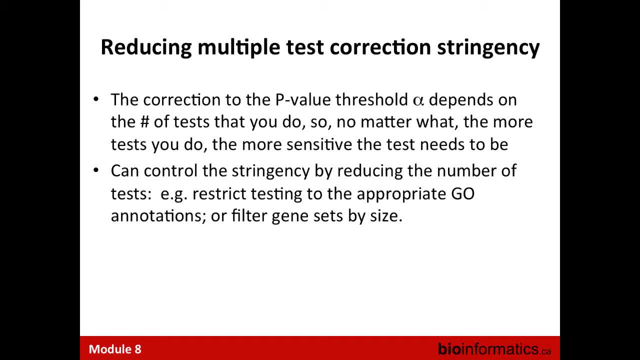 filter things out that you think are low confidence, and then you'll naturally have fewer tests to go through, and then each p-value will be considered more interesting as a sum. So one way of doing this is to filter in your input data. For example, if you are looking at gene expression data, 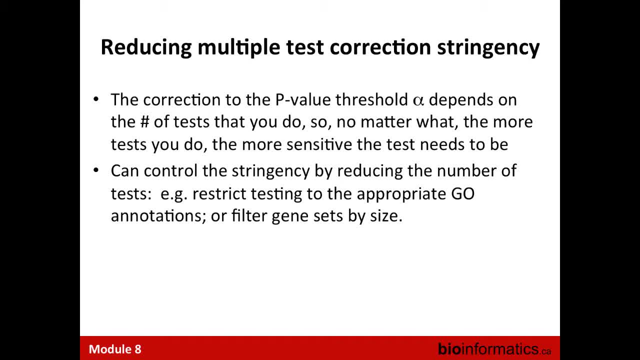 in RNA sequencing then quite often people filter genes that are expressed at a very low level. So because they're expressed at a very low level, you don't have very good confidence whether they were expressed or whether it was noise and you can filter them. 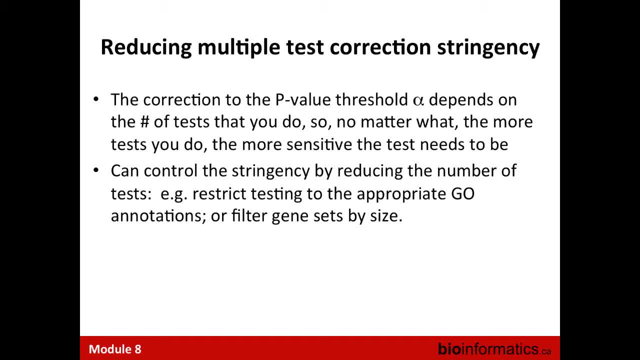 In pathway enrichment analysis, you may want to take a hard look at the pathways that you're analyzing. For example, there may be thousands of pathways that are just associated to one gene, because they are very specific And therefore you may want to ignore. 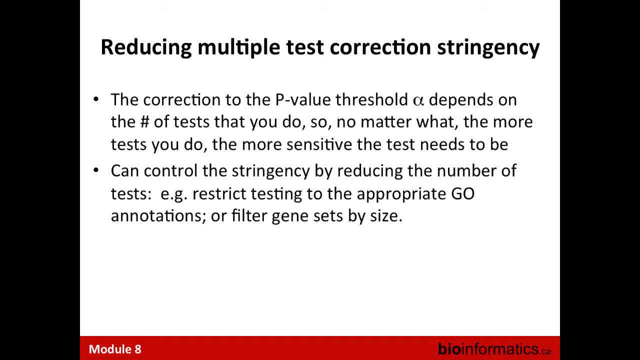 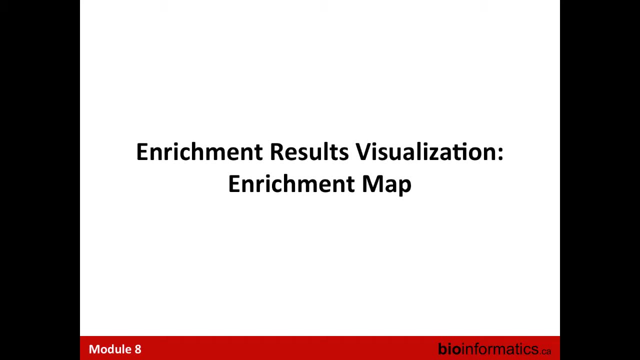 all these small number pathways and only focus on the larger ones. That will also dramatically reduce your false discovery corrections. So finally, once you have detected your interesting, enriched pathways, almost essential is the visualization of that data because, as we discussed earlier, there's a lot of redundancy. 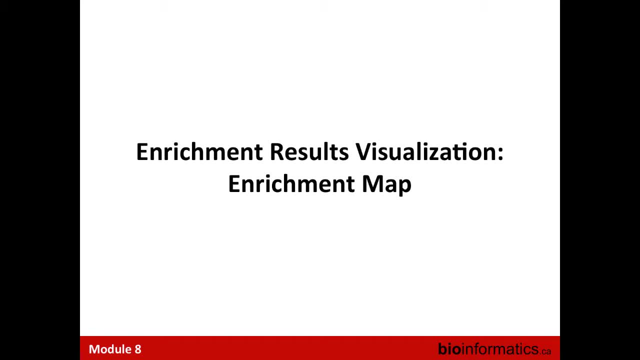 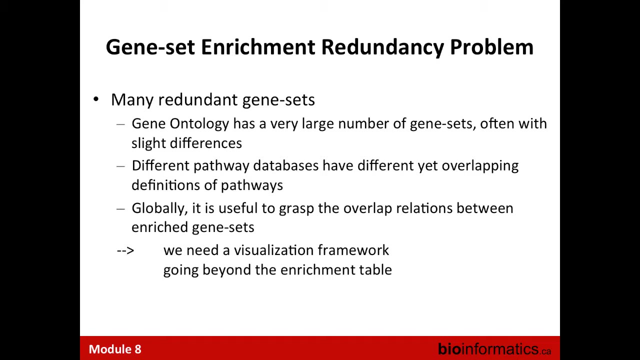 mostly because genes are involved in different pathways, but also because pathways are called different names and different levels of specificity. So one way of doing that is to build an enrichment map. The problem we already discussed: there are many gene sets and there are different definitions of pathways. 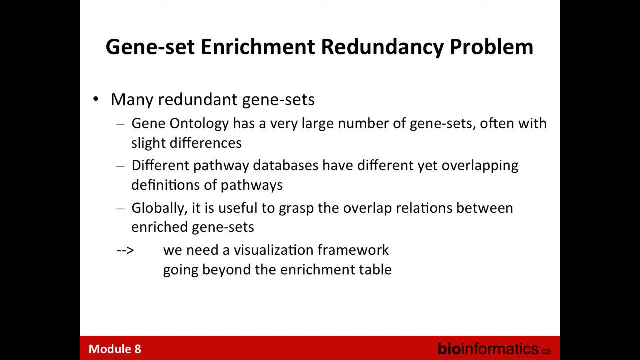 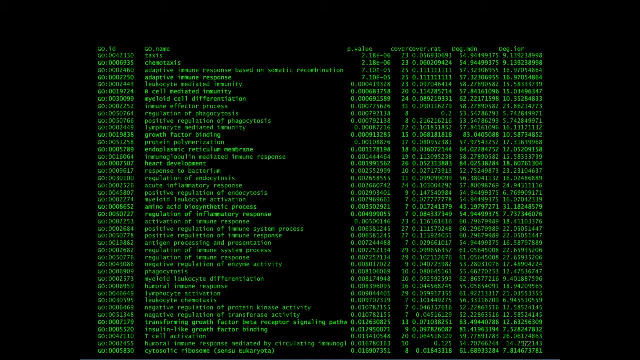 Moreover, when you start to analyze, say, two pathway databases at the same time- gene ontology and reactome- they will overlap by a large extent. So here's an example: You started by analyzing 100 genes and you thought that you can boil them down. 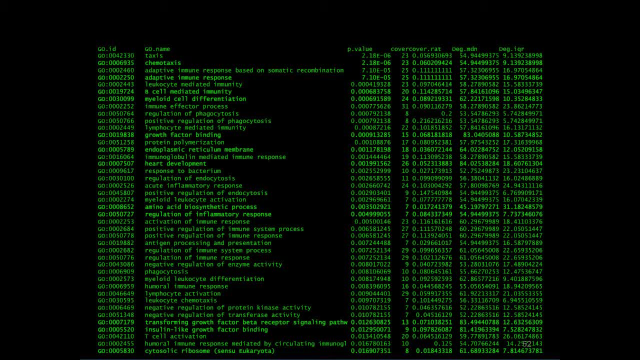 to three pathways, but it turns out that you boil them down to 500 pathways. What do you do? You can rank them by p-value and take the top 10 pathways, but because they're all redundant, it can turn out that the top 10 pathways 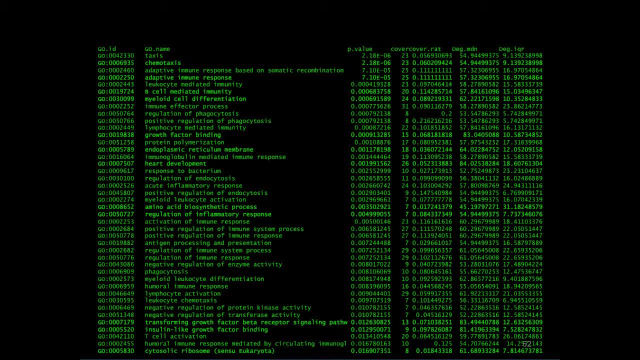 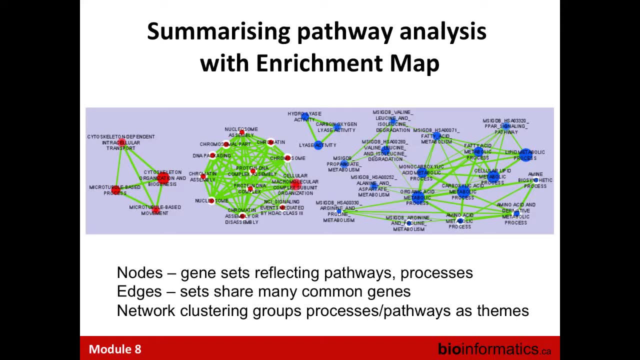 represent exactly the same thing that, for some reason, is quite strongly represented in your data, and the more interesting and non-redundant stuff comes down the road. The way we often visualize these pathway enrichment maps is called enrichment map and it's developed here at U of T. 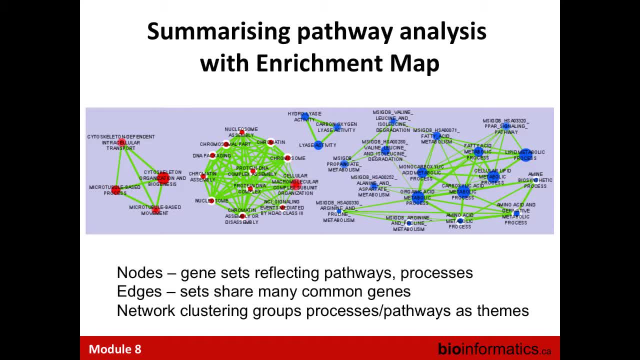 in the lab of Gary Bader. It's a network visualization, but as opposed to a classical network where genes are nodes and they're connected to other genes through edges, then this network is a network of pathways, So each node here represents a particular pathway. 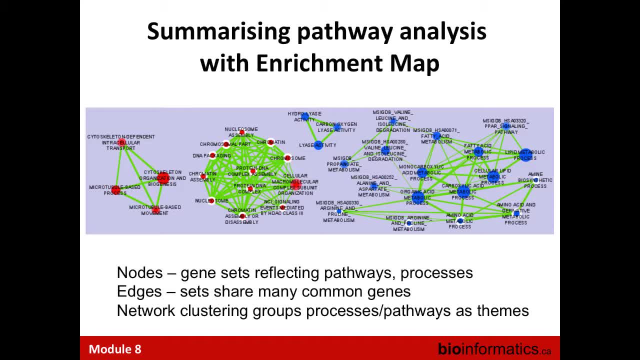 and it's connected to another node or another pathway if those two pathways share many genes. So if pathway A and pathway B share many genes, then maybe they are also functionally related or they're doing the same thing in cells, or maybe they're just two different descriptions. 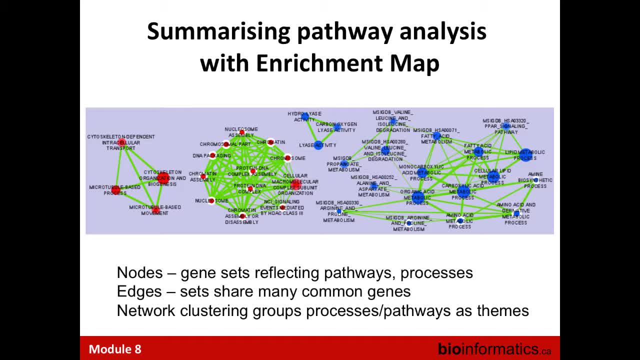 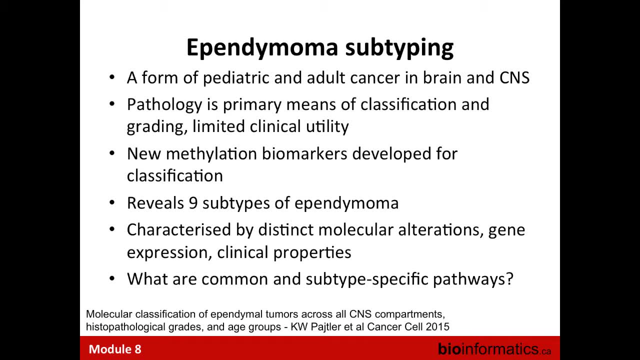 of the same biological phenomenon. One example of using pathway analysis together with enrichment maps in a nice way is coming from a paper of ependymoma. Ependymoma is a pediatric and adult nervous system cancer in brain and also the spine. Usually, pathology is the primary means. 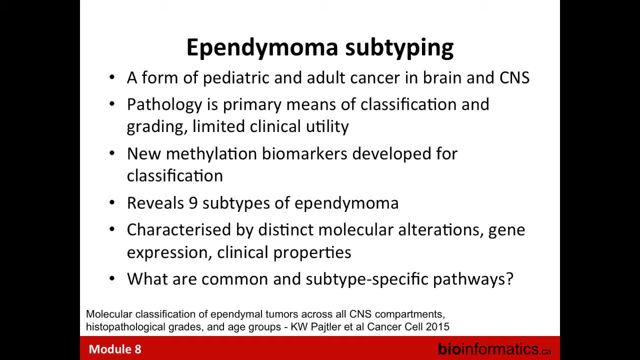 of understanding these tumors, which means microscopes and tissue slides and so on. However, now there are new methylation-based biomarkers developed for classification, And when you analyze these methylation patterns and gene expression patterns, it turns out that ependymoma is not a single disease. 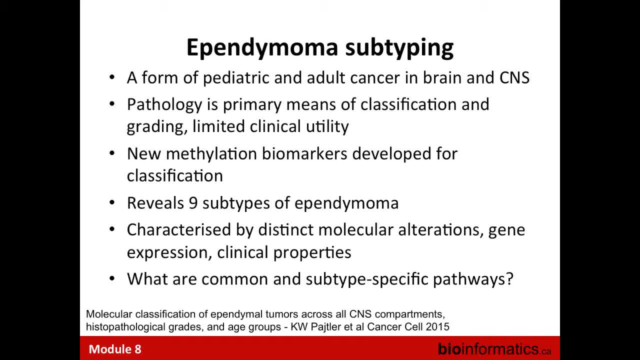 but it's comprised of multiple different subtypes which have distinct molecular alterations and clinical features and age characteristics and sex characteristics and so on. What we did in this analysis was to understand the biological underpinnings of these different subtypes using pathway enrichment analysis. 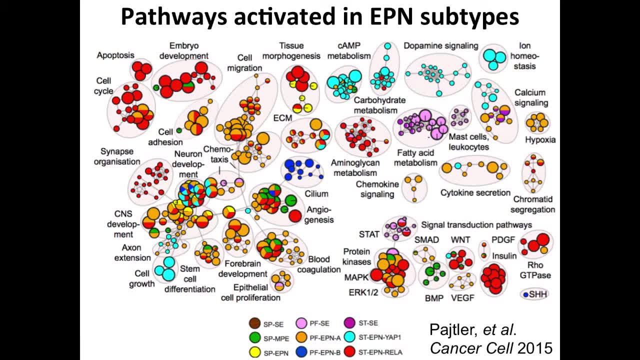 and network visualization shown here. In addition to highlighting these various pathways as nodes and as networks and clusters of pathways, we also used color annotation. Different colors correspond to these cancer subtypes of various kinds, And if a node has multiple colors assigned to them. 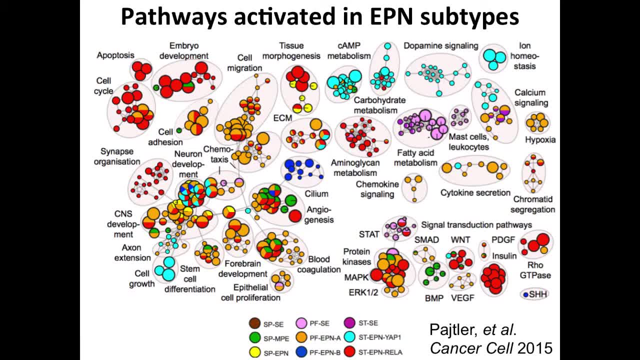 then that pathway is highly representative of multiple subtypes of ependymoma. So now we used to have nine lists of genes. Each one of them had hundreds or thousands of genes, And instead now we have dozens of biological themes that represent these nine lists of genes. 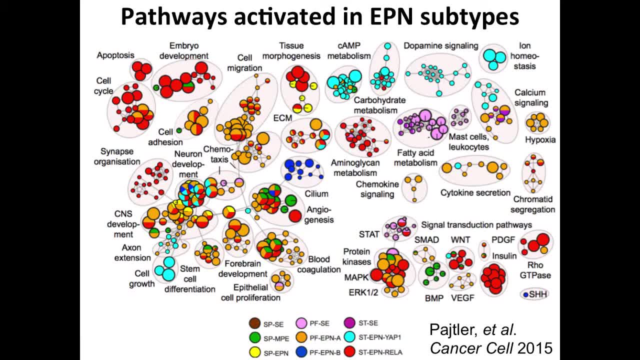 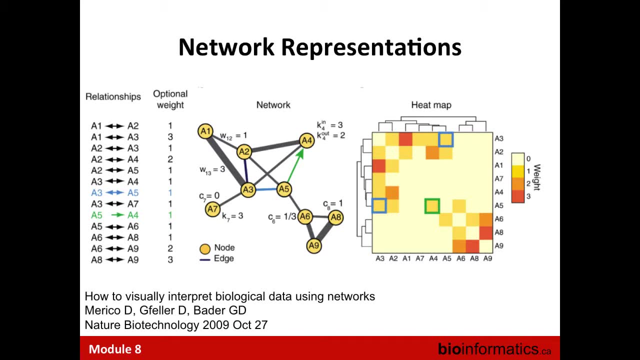 So we're going from individual genes to more biological interpretation, using textbook knowledge rather than alphabet soups of gene symbols. Okay, In the final chapter of this lecture, I'd just like to introduce a little bit of the Cytoscape software and about what it takes to build a network. 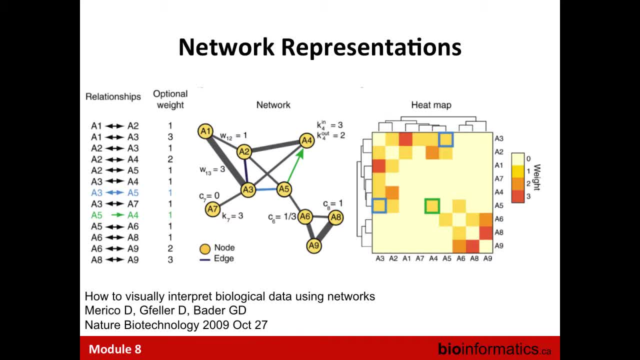 A network is ultimately a set of relationships, right? And you can build a network from just a very simple two-column table where the first column is node number one or gene number one and the second column is node number two or gene number two, And if they occur in the same pair. 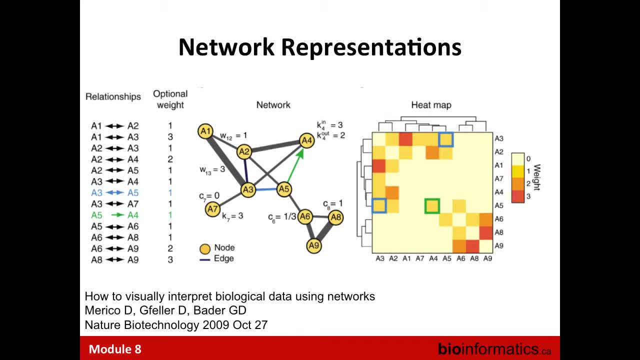 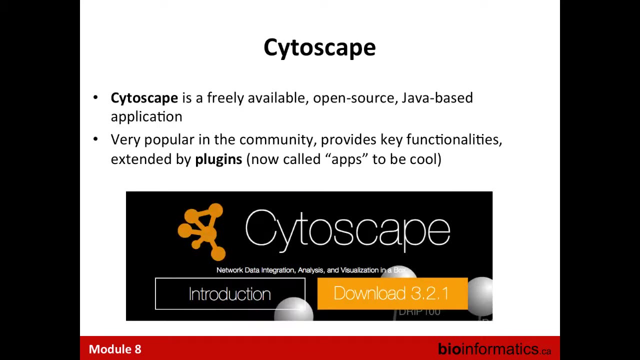 then they are interacting And you can generally assign a weight to any of these networks. And there are various ways of visualizing a network. You can also visualize the same network using a heat map, such as shown on the left. Cytoscape is a freely available open source. 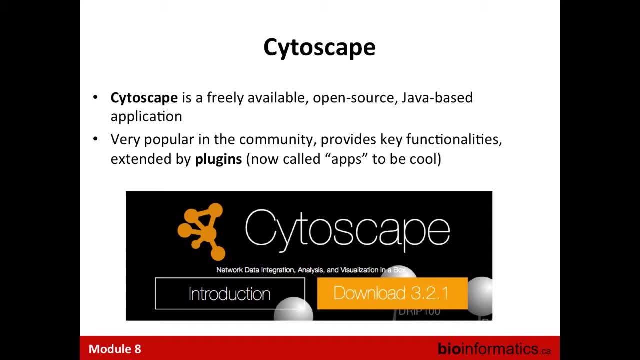 and Java-based application. In this tutorial that comes, we will use Cytoscape to build a network of pathways, but you can build a network of almost anything. One recent example is that you can build a network of wine-cheese pairings. 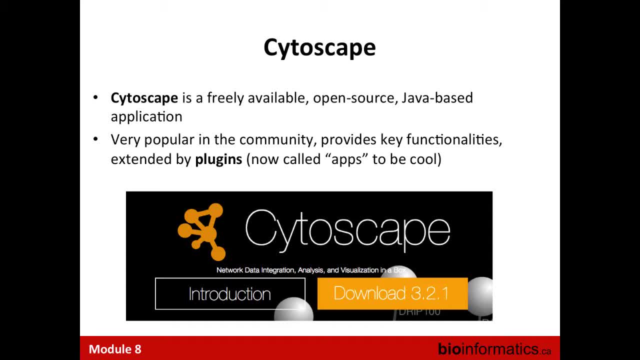 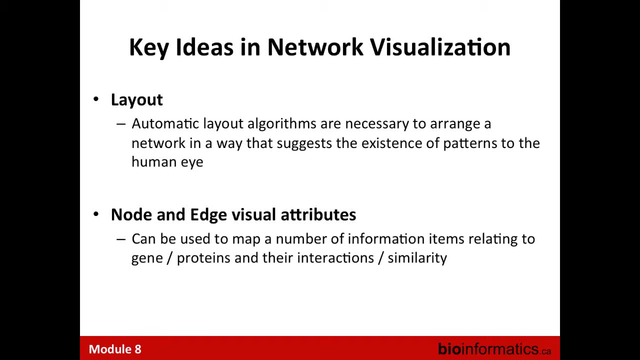 It was published by my former mentor, Gary Bader, just before the Christmas season, So it's a very powerful tool of visualizing knowledge and interactions. Some of the key ideas about network visualization: When you just build a network- and it's a large network- 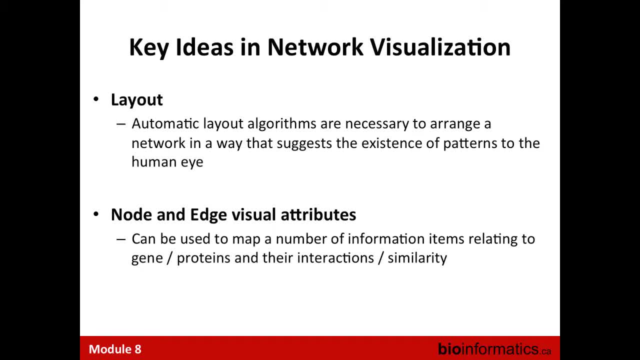 it will likely look like a hairball, Very difficult to interpret. So there's a whole battery of different network visualization tools that allow you to lay out the network in the two-dimensional and maybe three-dimensional space, and it becomes much more organized depending on these various network algorithms. 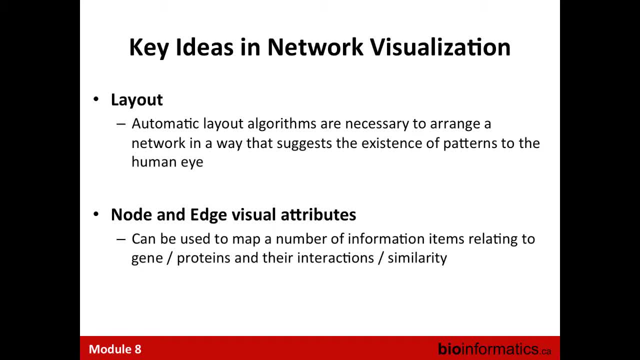 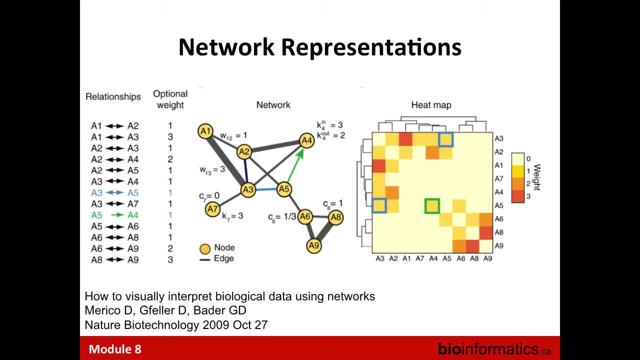 The other thing that Cytoscape is really powerful at is assigning visual attributes to your network. So, as we saw earlier, we have pairs of nodes or genes, and they're optional weights. You can immediately start to assign these features to your network. 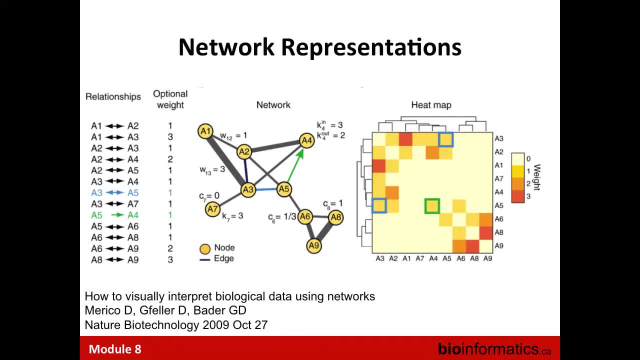 For example, thicker edges mean that there's a stronger interaction between genes. If a node is larger, maybe that gene is somehow more important or more central to the network, so on and so forth. There's probably several dozen of features that you can assign for nodes or edges. 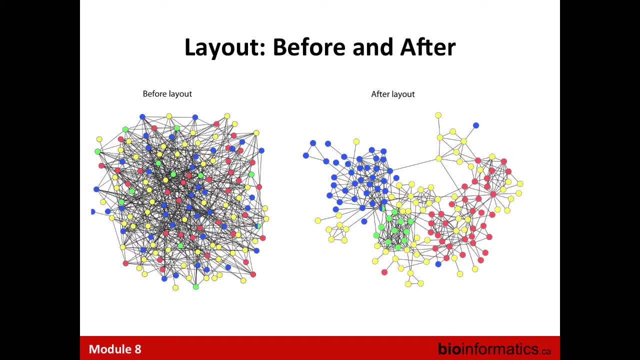 and it looks visually really appealing. So here's an example of a network layout before and after. When you're just loading your network into Cytoscape, it will look like a difficult hairball to interpret, but when you lay it out, 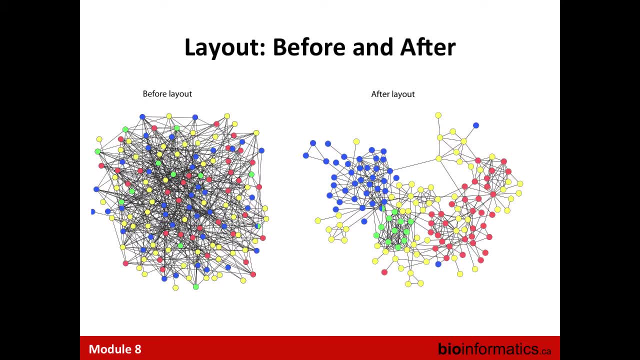 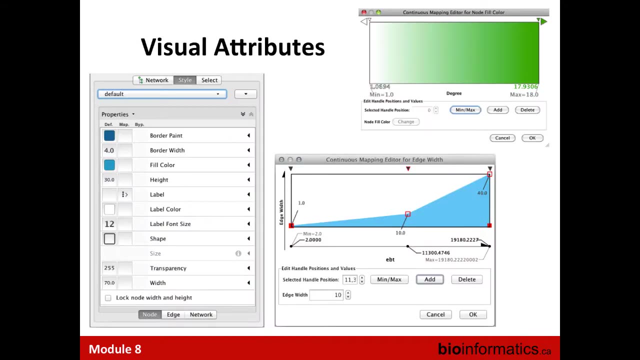 it starts to show clusters, Maybe all the blue genes are interacting with one another way more often than genes of different colors. And then you can start to build a hypothesis by just visualizing and looking at the data in various rotations. Visual attribute loading into the network.